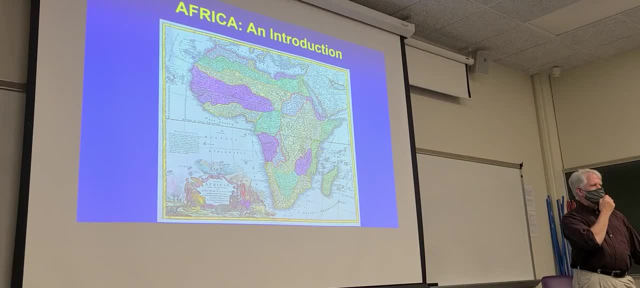 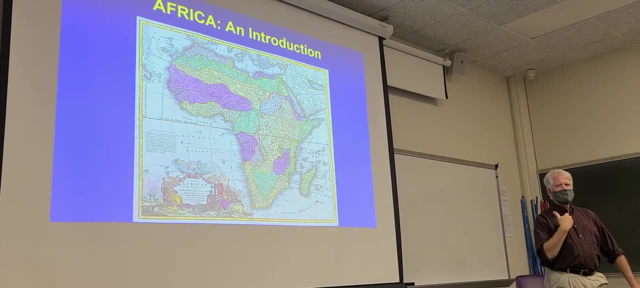 I teach again in the Department of Earth, Environment and Society. Some regulations for COVID regulations here say: you can take your mask off. If I'm far enough, I can take my mask off. Is everybody comfortable if I do that? No, I'm just kidding. 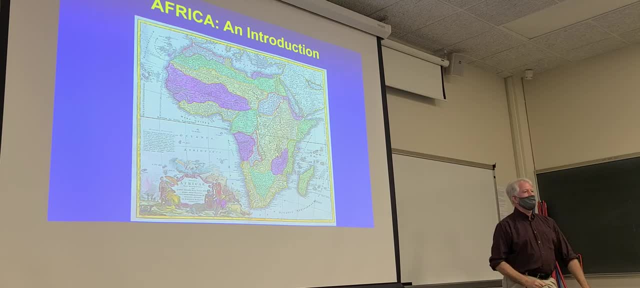 Oh, I was going to say, if anybody do feel embarrassed or anything, if you don't want me to take my mask off, I won't, All right. if we're good, let me know. I won't walk around. Well, like you maybe when I graduated as an undergraduate. 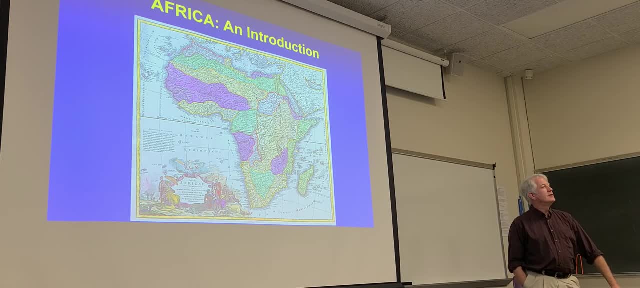 back in the dark ages, right 1981, I had a degree in biochemistry. So I went and I worked in a research lab after graduation in Connecticut, where I was on the fifth floor of a research facility trying to isolate the- it sounds exciting- the nickel-binding protein. 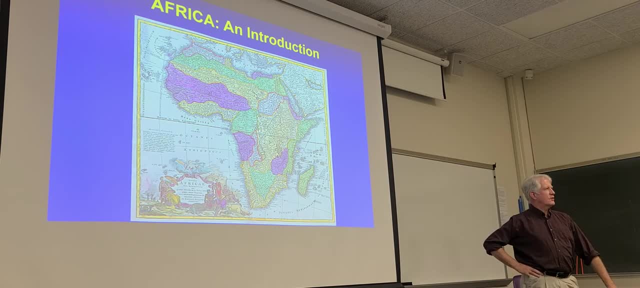 in the rat kidneys. I would inject rats with radioactive nickel, let it course through their system, cut out their kidneys, mush them up, put them through a scintillation counter and then HPLC to try to separate which proteins bound up nickel. 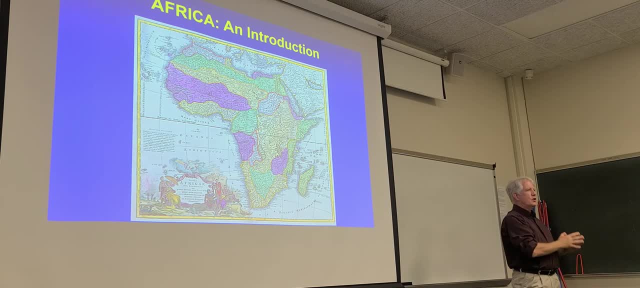 because we were studying a disease, Legionnaire's disease, and we thought that it was hypernickely too much nickel. It's about as exciting as you can imagine. In other words, not at all. White lab coats. what else it likes? 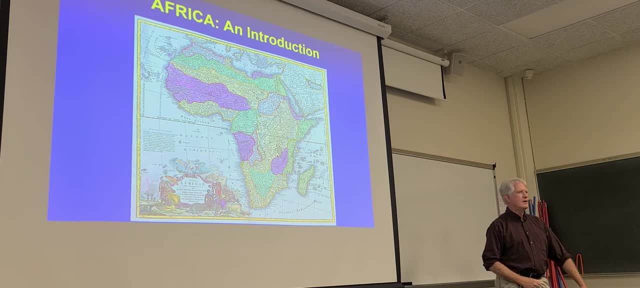 I did that for a year and I said: you know, this really isn't doing it for me, So you're like a mad scientist, So I what You're like a mad scientist. That hasn't changed. Yeah, it's still not. 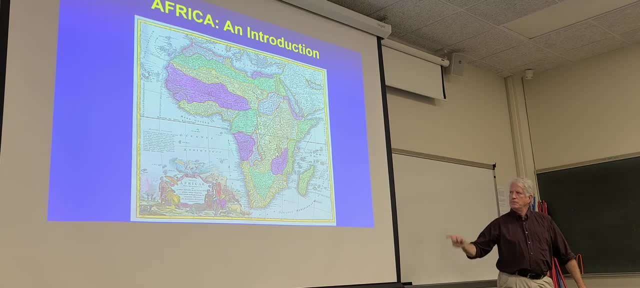 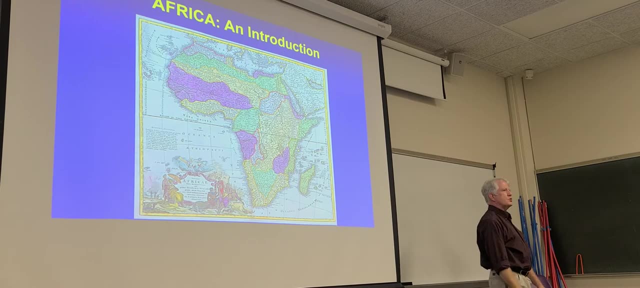 Totally pivoted and I joined the Peace Corps and I went to the Congo. Then it was called Zaire, but basically this region and through here, Democratic Republic of the Congo. they teach high school biology and chemistry in a small village in French. 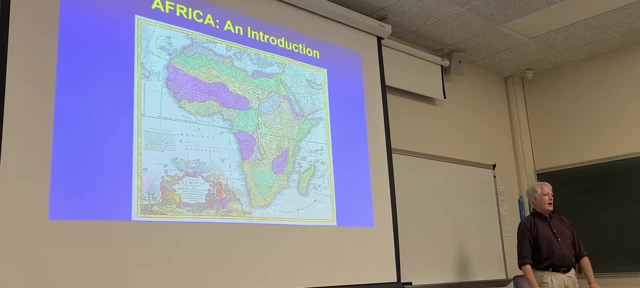 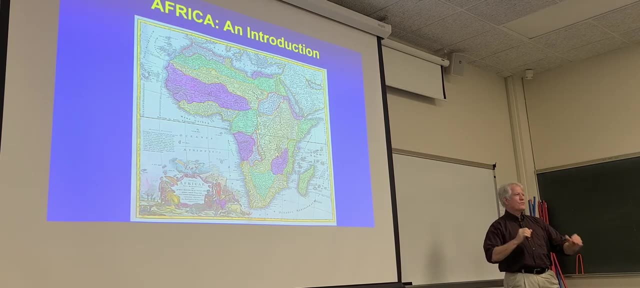 All right, so it's a training program out to the village. I was a skinny white guy from New England plopped down and I can still in my mind see the doors of that plane open when it landed in Kinshasa. 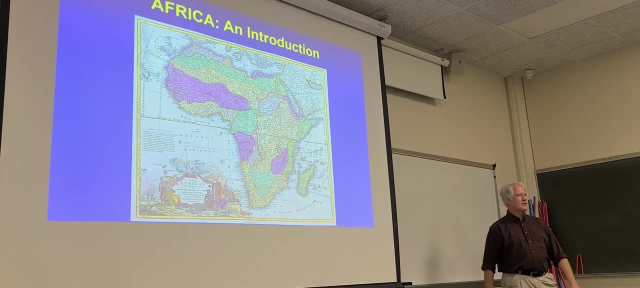 The heat that rolled off the tarmac, walking down the stairs and saying I'm in a totally different place than I grew up. right, All your anchors are kind of cut, Food language Everything. everything's different. So I settled into my small village of Gungu, in the region of Bandungu of Zaire. 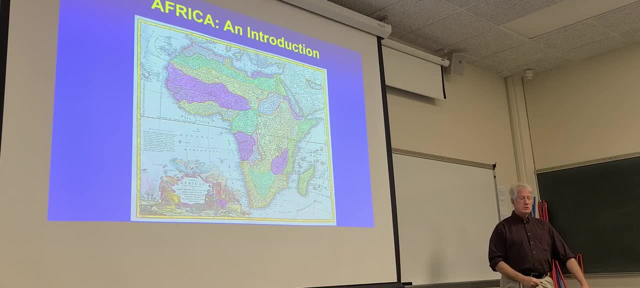 now Democratic Republic of the Congo, where I taught high school biology and chemistry for two years, And then I- you loved it or you hated it- I loved it, So I stayed another three more years there in different regions of Zaire. 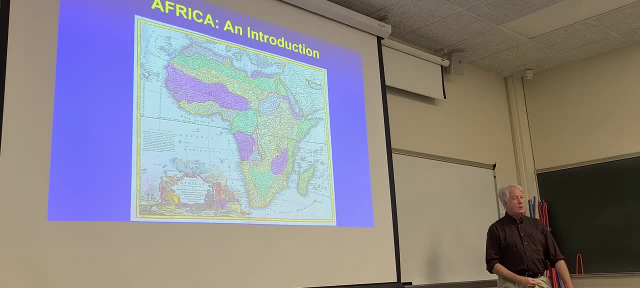 working on other development issues. What I found was while teaching kids how to use a microscope and biology and chemistry so they can pass their high school exams, which was important. some of the basic needs were more in agriculture- food production. So I came back, got a master's degree in agronomy in California. 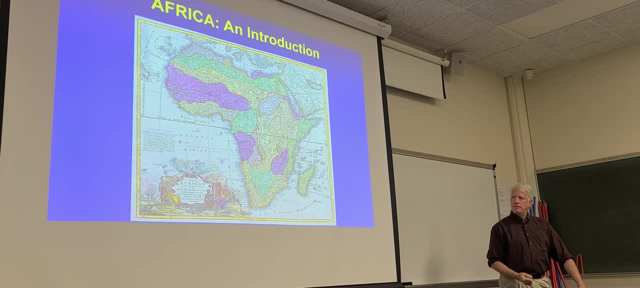 and went back for three more years working in Senegal, West Africa, Botswana- a couple tours in Botswana, Burundi, Cameroon- So these were parts of sub-Saharan Africa. So what I'd like to talk to you today is just an overview about my impressions of Africa. 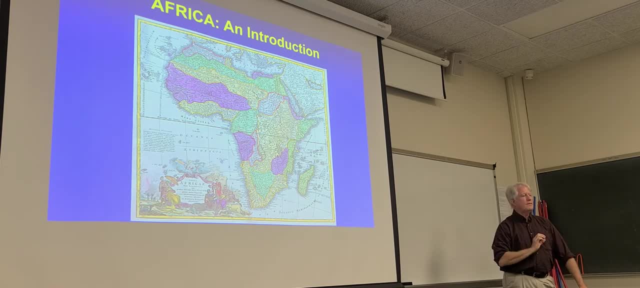 in just a few minutes. Thank you. Different segments, right? So some of this is going to be about population growth, perhaps unique health issues that they face- Recent scares with Ebola, for example, that you may remember Some challenges that they have that are not unique to Africa, but maybe some that are. 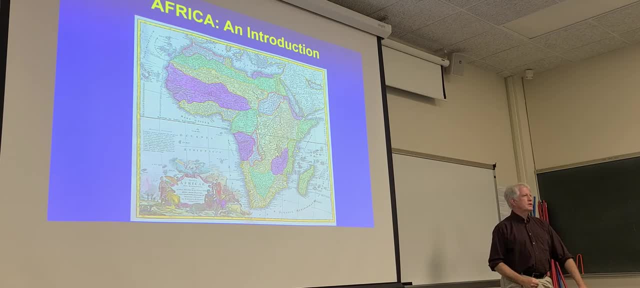 And as a world community, how should they be addressed? Because the UN is very cognizant of pulling up less economically developed countries to get them more developed and self-sustaining. So has anybody here? is anybody here from Africa or been to Africa? 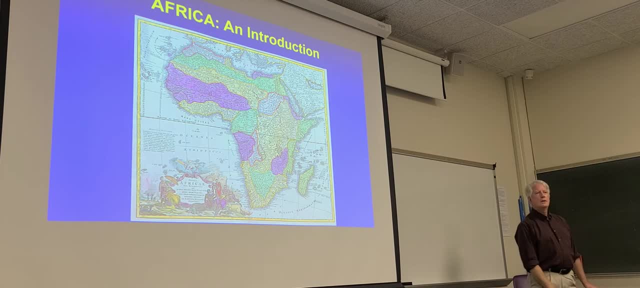 I'm from Africa. Where are you from? I'm from East and North Africa. East and North. yeah, This is an old map. Let me get a more modern map. I'll get a modern map in a second. Anyone else from Africa? 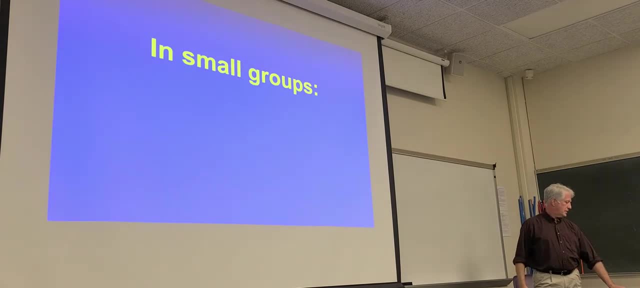 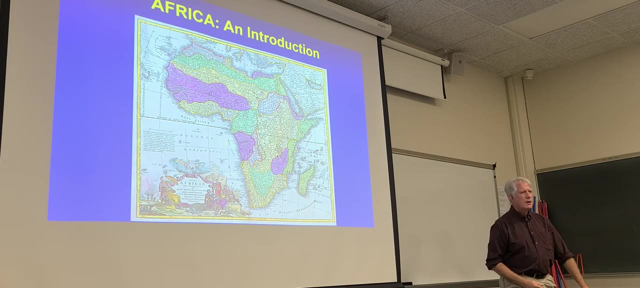 We're not from Africa, but I've been to Africa. Yeah, You've been there. Yeah, Where have you been? I've been to Kenya and Somalia. Kenya and Somalia- Yeah, You've been there. Yeah, Where have you been. 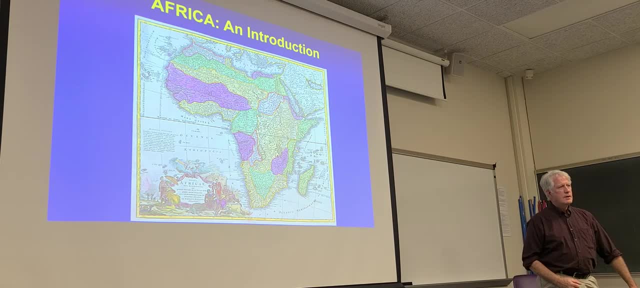 I've been to Kenya and Somalia. Kenya and Somalia. Yeah, I've been to Liberia, Liberia west. Oh, Ethiopia, Where Ethiopia? Ethiopia, okay, And where else Anybody? There's some great study abroad if you are interested. 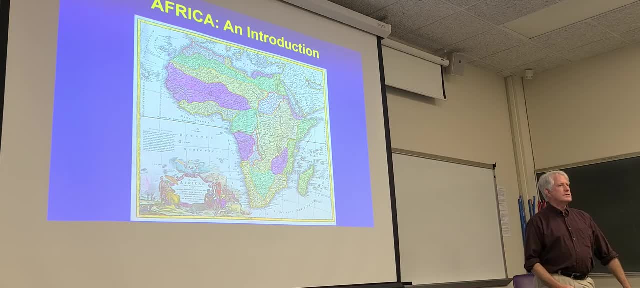 Senegal is just a magnificent place. Ghana, again, a very magnificent place to get the opportunity- Many other you might go with your family, or the opportunity to go on a safari or something like that. But there are some challenges in some places that are. infrastructure is tough and maybe 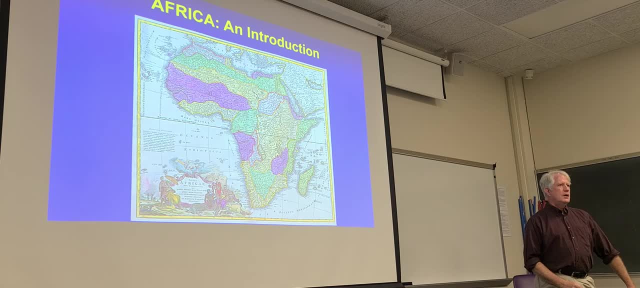 some political situations are a little less stable, but I don't want you to come away with the impression that many people have that this isn't a nation, that this is a country. Many people, when I came back, said, well, say something in African. 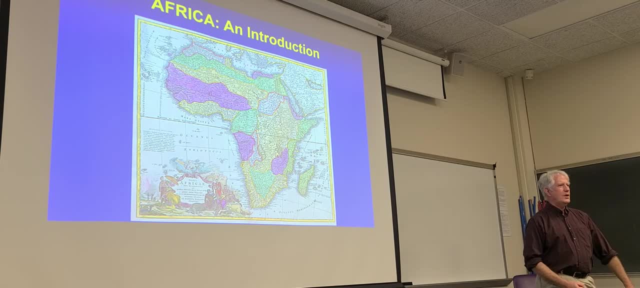 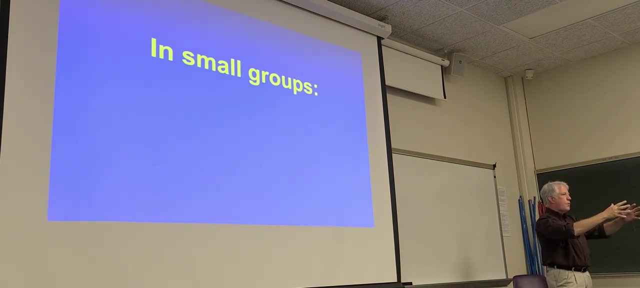 It's like say something in European. I mean, what do you pick? right? This is, every country is different, has their own unique governments and challenges, et cetera. So with that, just maybe five minutes, small groups get into like four, you know, groups. 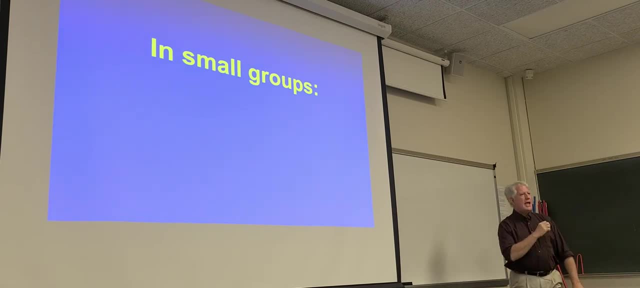 of four or so if you want to wheel yourself around and come up with a list of everything that you know. when somebody says Africa, everything you know about Africa, all your preconceptions, let me put it that way. So why don't we do that right now? 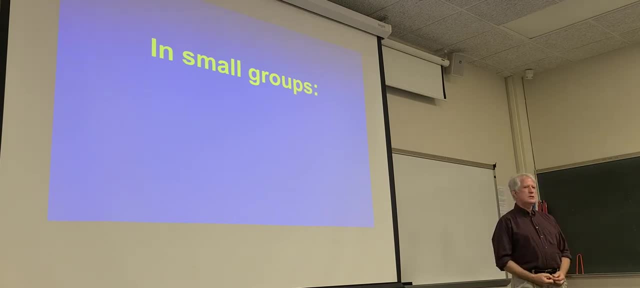 Just circle the wagons and just take five minutes. Three, two, one go. Okay, I believe it was like. what are your impressions of it as a place overall? 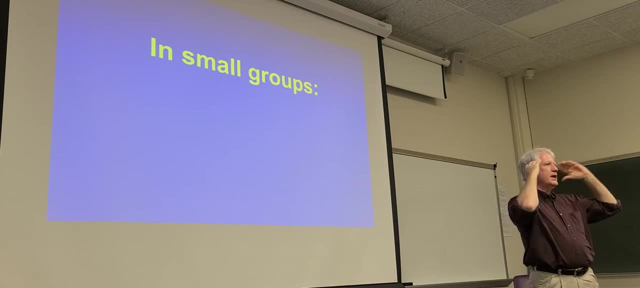 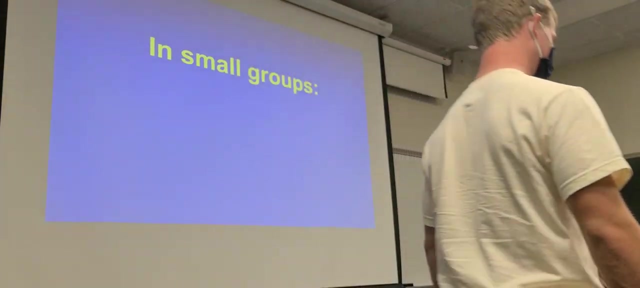 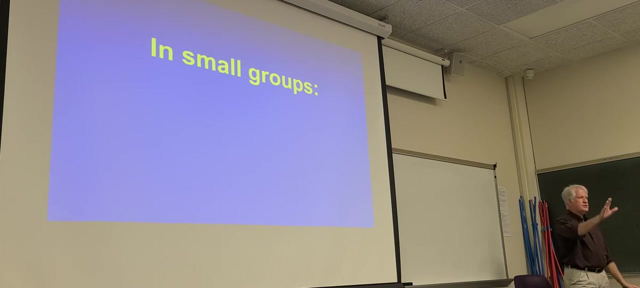 Yeah. when somebody says just Africa, what do you think of Like? what are the preconceptions or the ideas that come to mind? I guess? Yeah, I do too. Thank you, My first impression was: hot, Hot. 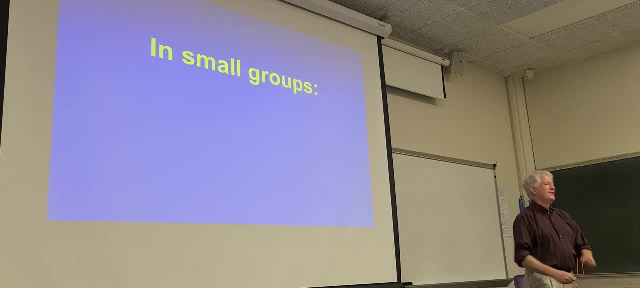 Hot, Hot. I was going to say pot. That's Colorado. How about you guys? back there, Our first impression was like: we think of natural resources, We think of wealth, We think of you know everything that Africa has naturally. 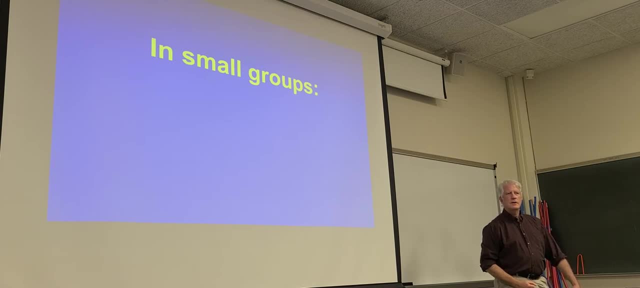 And then we said we thought about how sometimes we think of chaos or whatever, just because It's hard to control everything that they have there and keeping everything they have there. But we thought of it as a beautiful place for the most part, Yeah. Yeah, There's a lot of natural resources. Yeah, Some. But you know, if you look at the United States, it's not all centralized either. I mean, you go to the southwestern United States, it's pretty much a desert. 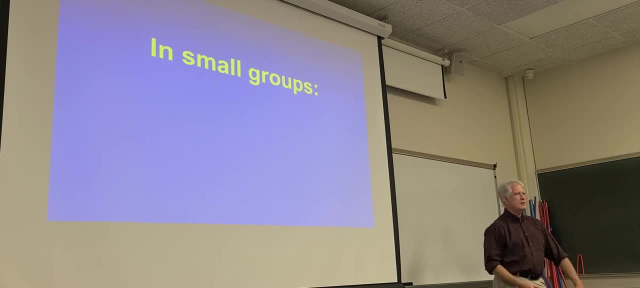 The scarcity is water. That dictates it right. And then you go up to the, to Iowa, and they got corn, as far as I can see right. So the same thing with Africa, It's like anywhere else. There are some countries that just 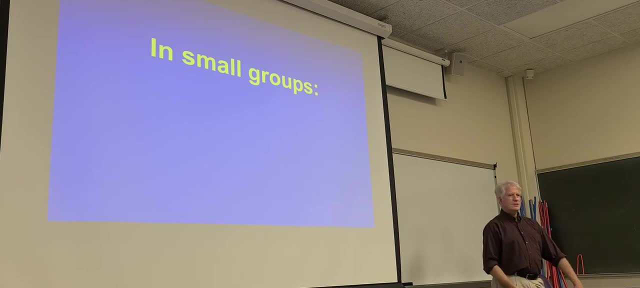 Luckily there are borders. There's, you know, gold, You know there's. there's much of the rare metals that are in your cell phones now come from Democratic Republic of Canada and some other places. It's not equitably distributed throughout the population, but the wealth 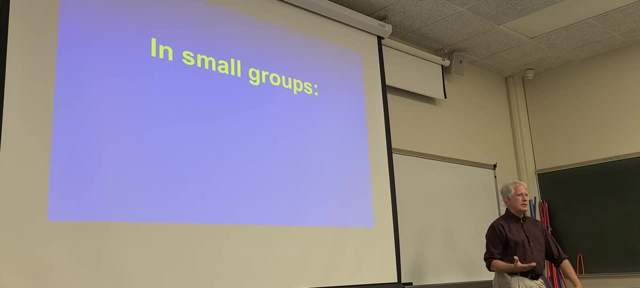 But some countries just have a port, Other countries are landlocked And this is kind of like like everywhere else. Right, Don't think of Africa as any different than anywhere else. It's just about its distribution of potential, I guess. 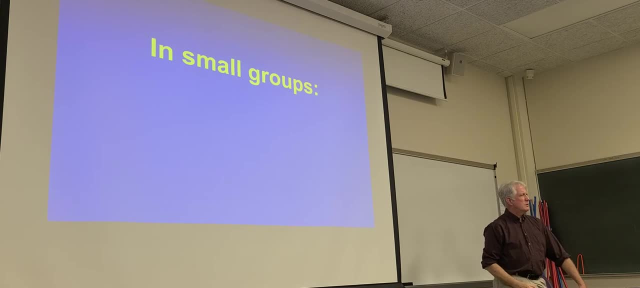 Back here, Not even the Nile Right, Not. Is it like flies the safari? Not safari Everybody thinks of, like safari or jungle book or Tarzan or you know those. you know that kind of stuff, But certainly you know the pyramids, the iconic tourist destinations. 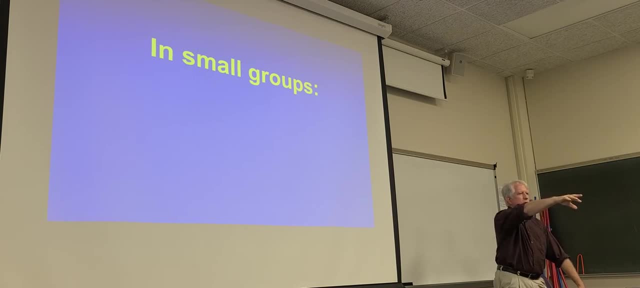 How about your group here in the middle? You know they talked about how massive it is and how difficult it is to traverse it all and how diverse it is, and like how many different climates there are. Yeah, that's a good one. Climates. 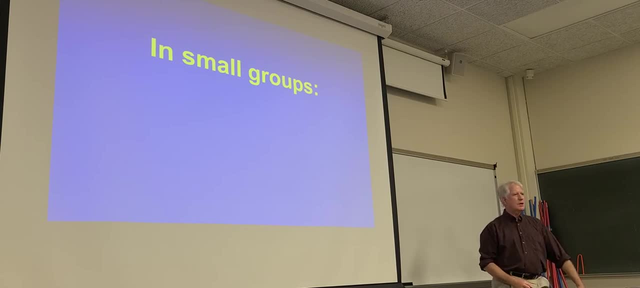 Because climate is what you get. You really can't change it all that much, So that dictates it. So one of the, you know, the biggest rainforest or jungle in the world, Amazon Right, The biggest river drainage in the world, Amazonian River west to east into the Atlantic. 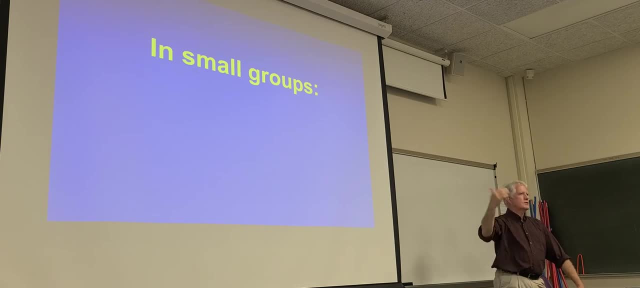 The second Congo Right Rainforest, and then the Congo into the Atlantic Right, Second by discharge. So it sits on the equator, That's the climate And we'll leave that there. So I want to pick some of this stuff apart. 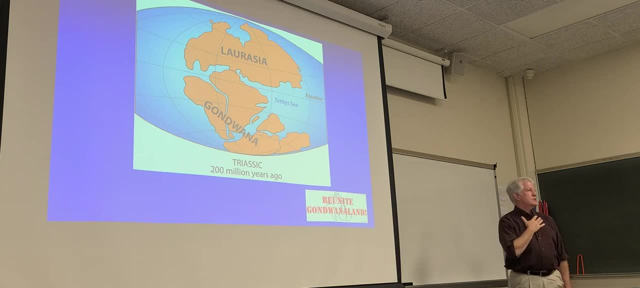 Now again, this is. Some of this is just demographic data, Some of it is my impressions. It's an old continent, All right, So if you think about it, it hasn't moved that much over the millennium from where it was kind of started. 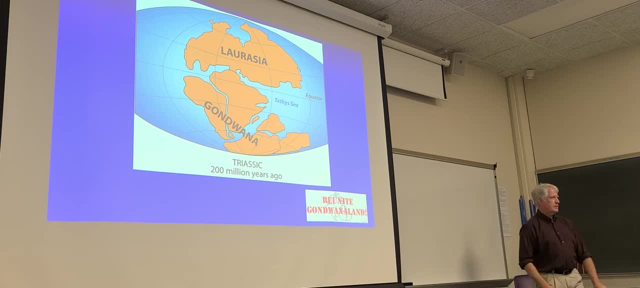 India took a great tour Right. It went clear up and still slamming into the belly of Asia, pushing up the Himalayas. But Africa is an old continent, So it's been rained on a lot And I think that's a good thing. 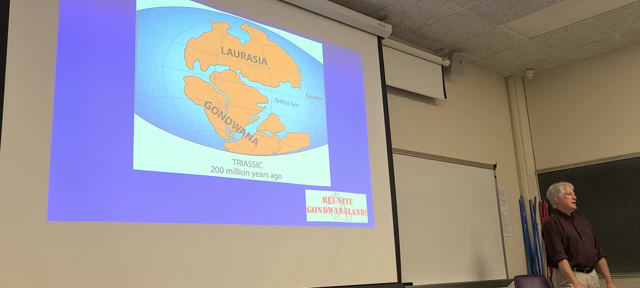 I think that's a good thing, And I think that's a good thing, And I think that's a good thing, And I think that's a good thing. It's been rained on a lot. It has been sitting there a long time. 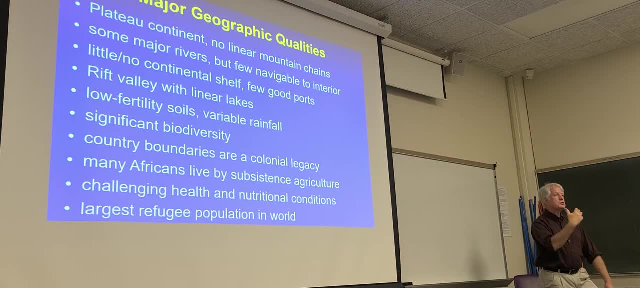 So fairly intact, Which gives it, imparts to it, certain geographic properties. Right, So this is a geography course. I'd like to start by just what is the physical geography of Africa? All right, They have some pluses and minuses. 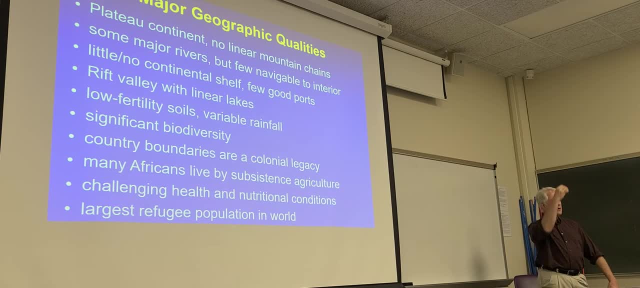 Minus: no long linear mountain ranges. They have volcanoes Right, Some dormants, But think of Mount Kenya, Mount Kilimanjaro, Right, And you can see that there's a lot of land. they have rift valleys. in other words, some of it is still tearing apart right, kind of like the red. 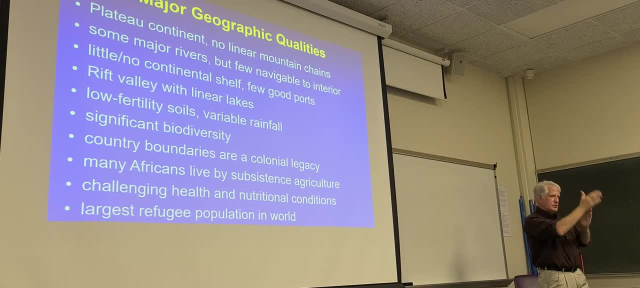 sea. it's pulling apart a little bit. you have these long linear lakes. it sits on the equator, which means it rains a lot there, and then about 30 degrees north and south of that is pretty dry. so you have the saharan desert. that's not small. that's about as big as the lower 40 united states. 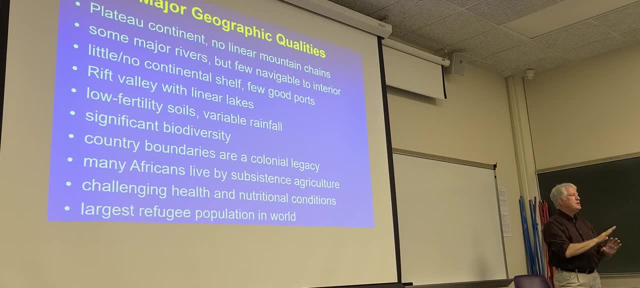 right. and then you have down, you know, botswana and namibia around that area, that you have in kalahari right. so this dictates a lot of different things. um, in the past, one of the best ways to get into the interior and for trade is by rivers right. most cities of the world develop on rivers because 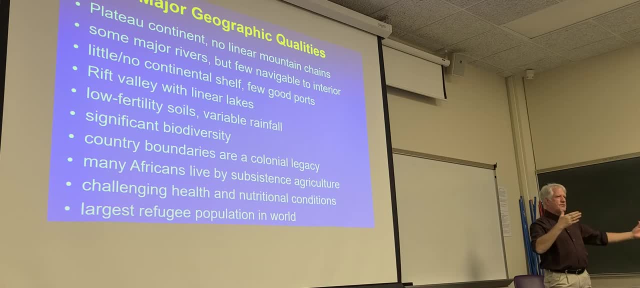 it's a great transport to the interior. it's defensible, right, you live on one side. you've got a river as a boat on the other side. it's great to get fresh water coming from one side and throw your waste down the other side. unfortunately, africa doesn't have a lot of navigable rivers from ocean to the interior. 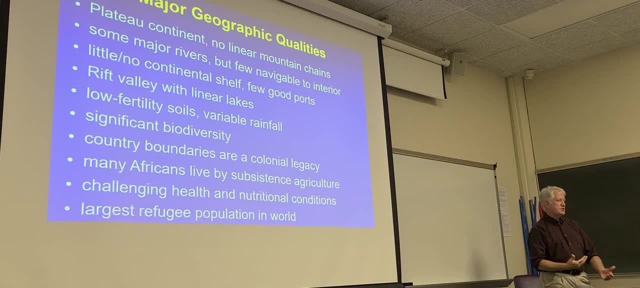 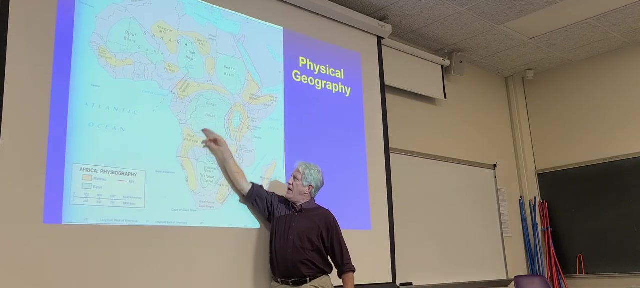 right. i'll get to that in a second. so it has some challenges maybe some other continents didn't have. but it has other challenges as well that other continents didn't have- think colonialism, slavery. but this is the physical geography of africa, so this equator right drains most of the congo basin. 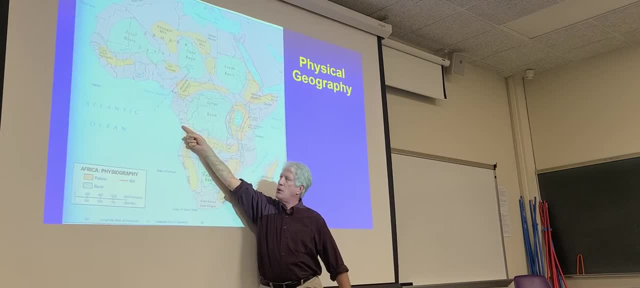 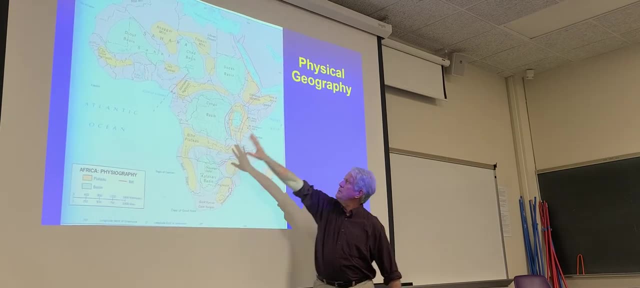 is raining somewhere here every day, which means a lot of water being pulsed out through the mouth right of the congo or the zire river into the atlantic. there's a kalahari basin here, chad basin, the basements in the north, and those are. those are fairly dry, so there's no long linear. 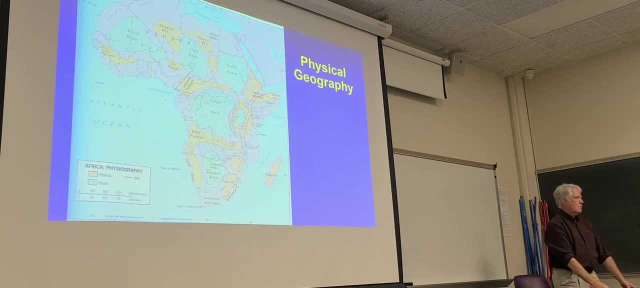 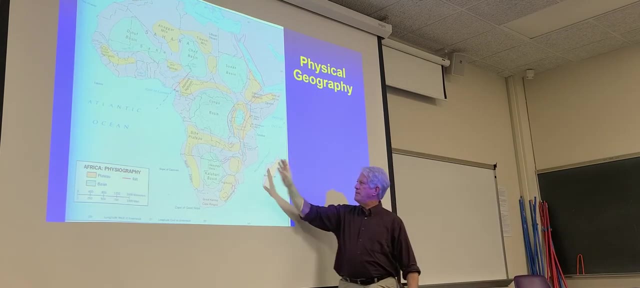 mountain range, like the andes in south america or the himalayas or something like that. it's a little more spotted. this is that crack- so postulated madagascar cracked off and you play tectonic movement and that the same thing is happening here. these long linear links. 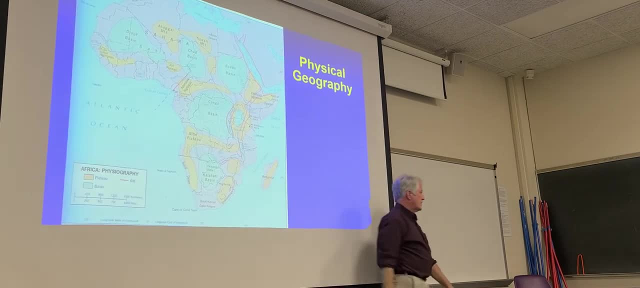 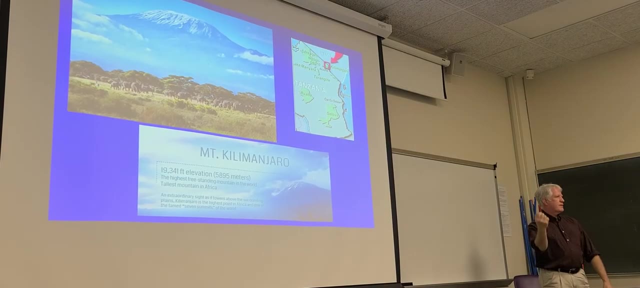 right, happened up here in the red sea, but now this is starting to separate one of the great wonders of the world, that's one of the world. you've probably heard of: the lake of mount kilimanjaro, the snows of kilimanjaro. right, it's a mountain that kind of sits alone, but it's snow capped and it's on the equator. 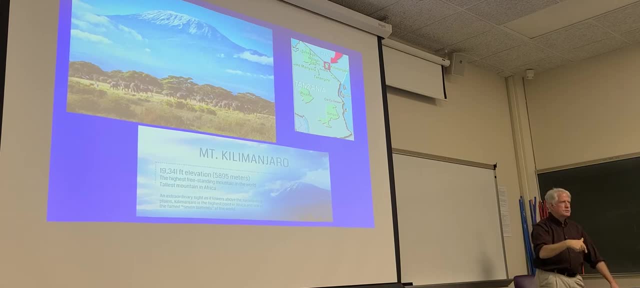 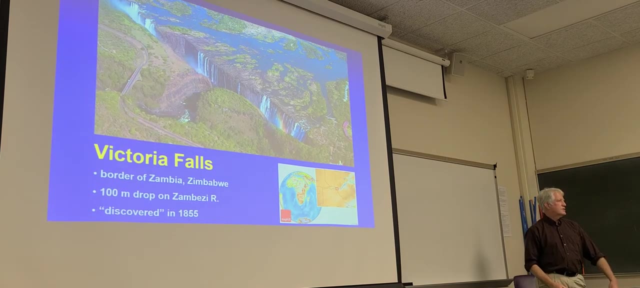 right. so that dictates a lot of the microclimate all around that one particular place. here's another great wonder of the world: right, big fall, victoria falls. people spend a lot of money to go to see if it falls right and you can do goofy things like you can. you can go kayaking that. 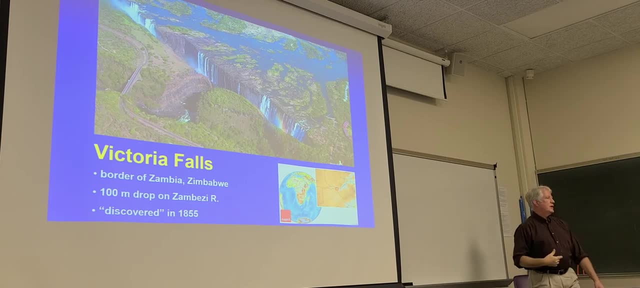 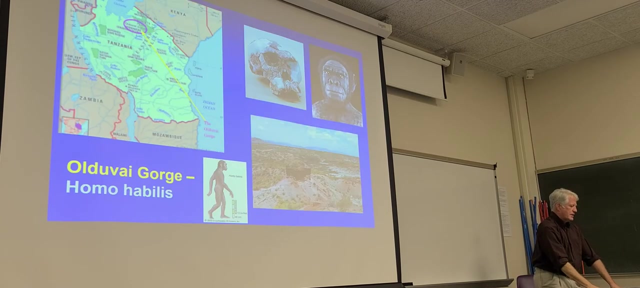 bridge right there you can go bungee jumping off of. in the past, i mean like 20, 30 years ago, if you did it naked, they give you, let you do it for free. it's like i don't know. i don't want to see anybody hang upside down, but a tourist you can fly over and help out and stuff like that. 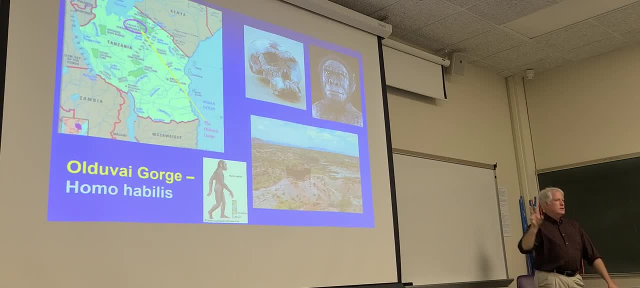 and then maybe another thing you've heard about africa in the media is origin, right origin of the asians here. homo habitus, so genus homo. we are genus homo sapiens. that was thought that this guy right walked out of africa back at a time when it was somewhat hospitable. 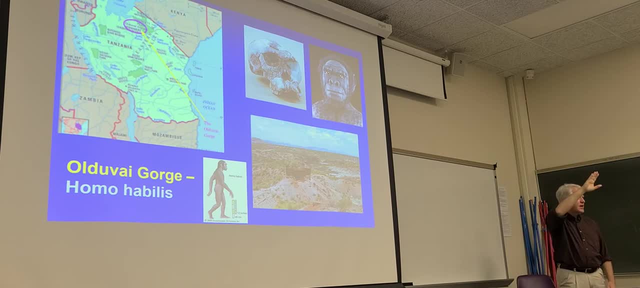 to pass up through, maybe, the nile track, but up through the sahara to europe. homo habilis, some stayed behind, some walked to europe. those ones that ended up in europe evolved. homo neanderthal, insist, neanderthals right, the ones that stay behind homo sapiens. and then they. 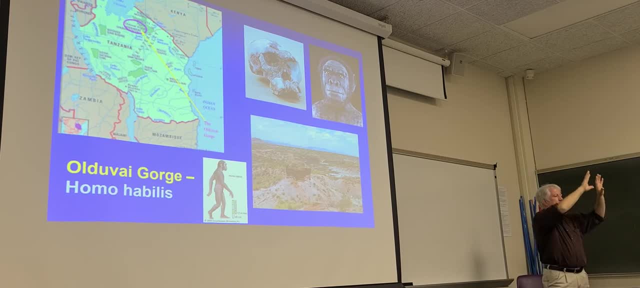 left africa, came up to asia, come up to europe, met neanderthals in europe. if you are from european ancestry, you probably have one or two percent neanderthal dna in you. if you were from african ancestry or asian ancestry, you probably don't. yeah, so how do we know about all this? well, you, 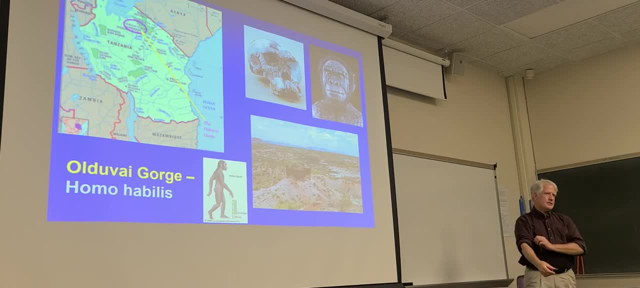 can take a whole course in this through artifacts. you can take a whole course in this through artifacts, right? so some of it's logical. in other words, if you were small and tasty and you didn't have claws or fangs, you needed protection. protection comes either from back up in the trees, right, but also. 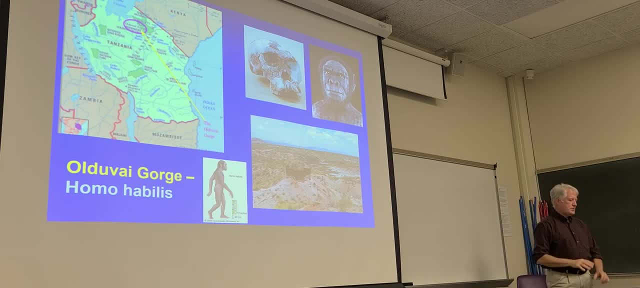 from groups, right? so if you stayed in groups and it's thought that these groups developed in this transitional zone of civility and then they developed in this transitional zone of civility, but then they haven't got claws or fangs, you can take a look or you know some of these femurs. 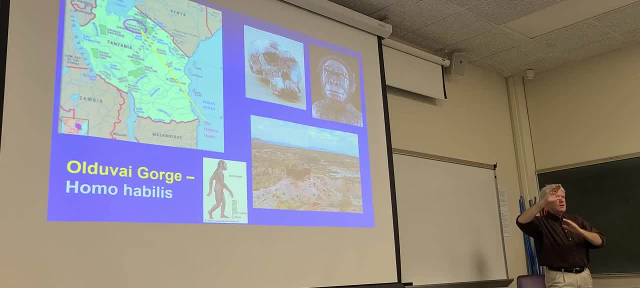 they can add a fang or an animal- the last thing we know about vana. so thorn tree grasslands. so the trees go back for protection. the grasslands to follow the herds. if rains come and go, you're following those herds with. you know that's your food supply. if you want to travel fast, go alone. 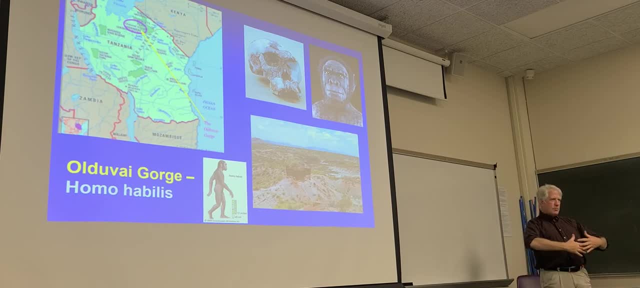 if you want to go far, go in a group. so if you look at other pre-hominids, they're usually much more able to get a mixed diet. we're able to slim down, lose the big belly, be more upright, walk, travel farther- right. so these guys eventually became beachcombers, right. so if you look at the diaspora, 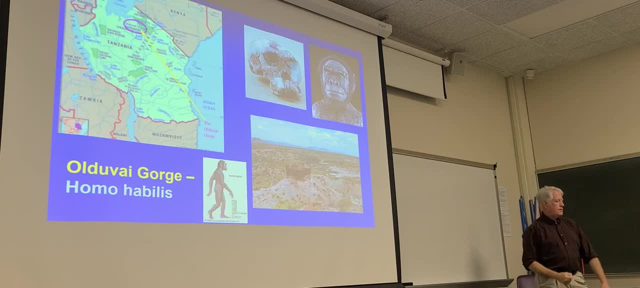 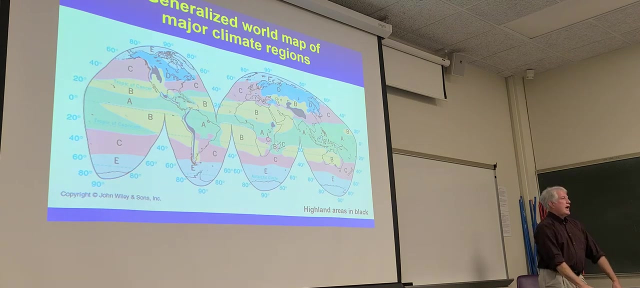 out of africa around the world of hominids anyway. usually they follow the beaches. that was the best place because a few things to eat you and a lot of things for you to eat, so not as many bone fragments and things like this. but they can't trace and date other types of artifacts, so out. 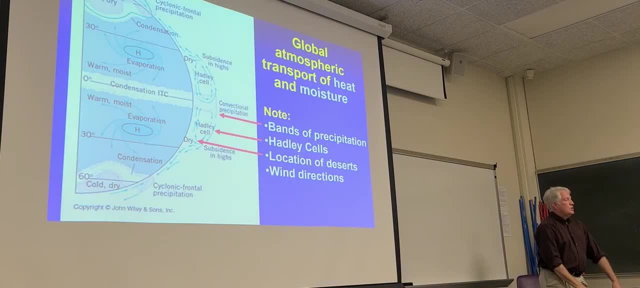 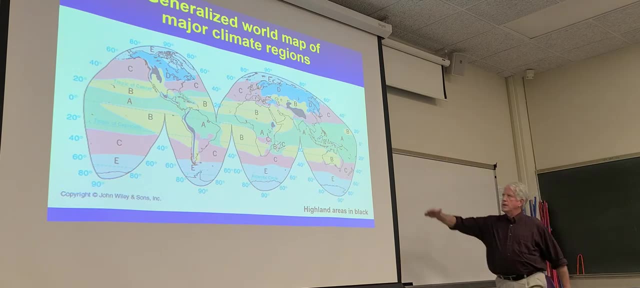 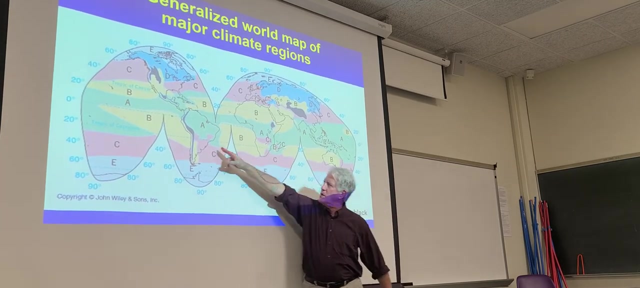 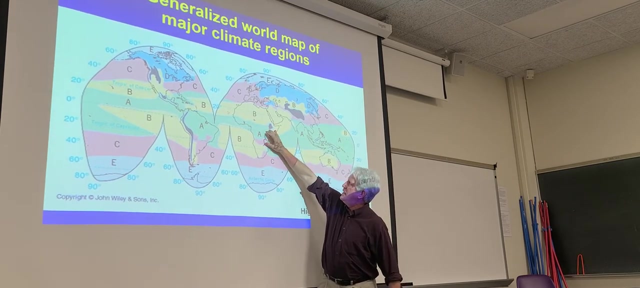 of africa? um, what makes africa maybe, unique, unlike other continents? if you look at the world, most land masses are in the northern hemisphere, not the southern hemisphere. those are in the northern hemisphere, usually have mountain ranges right which mess stuff up, except for africa. so it's poster child forward: always wet, always hot, drying out, and then at the ends you have more of a. 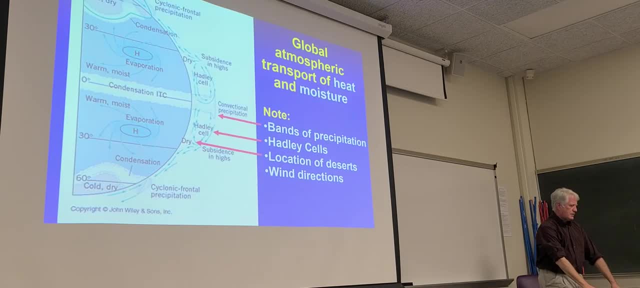 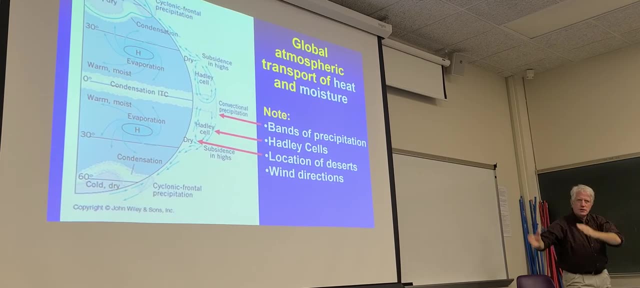 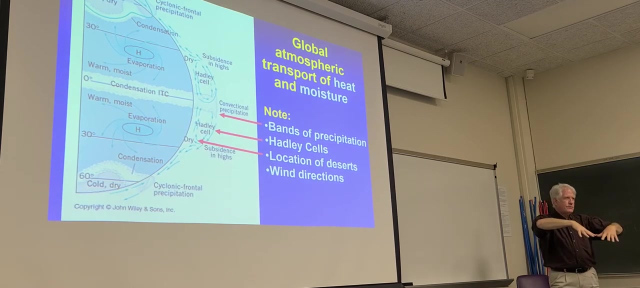 mediterranean climate, so it's kind of the perfect climate model. this is why there are deserts: 30 degrees north, 30 degrees south. heating at the equator, hot, warm air rises. as it rises, it cools, drops the moisture right back down where it got it from. your rainforest is there at the equator. 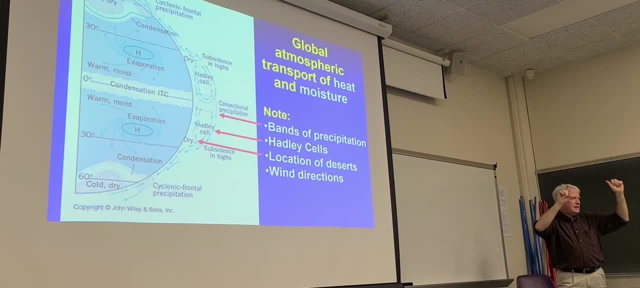 but now that air at the upper altitude is hot but it's dry, it moves forward and descends like a hair dryer on the surface, about 30 degrees north and south right, desiccating that surface, and it doesn't rain all that much. so this is why about. 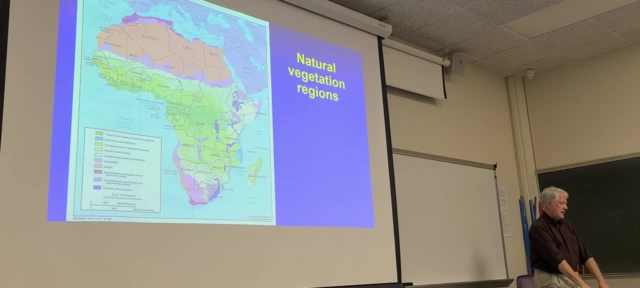 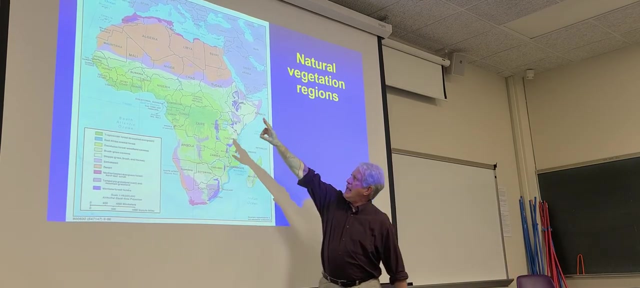 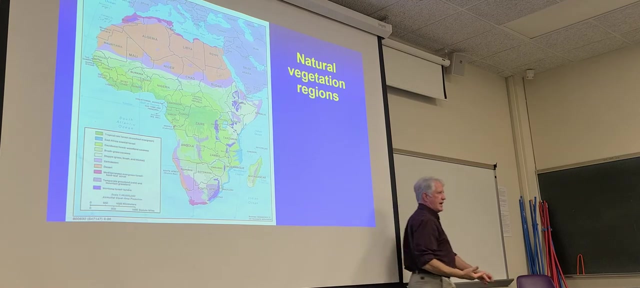 30 degrees north and south, you have these major deserts in africa. that's just geography. same thing here you have rainforest drying outs and bands as you move north and south. all right. so those countries that are maybe established in landlocked, no ports, no major river systems, in dry areas, cannot just like animal. you know just. 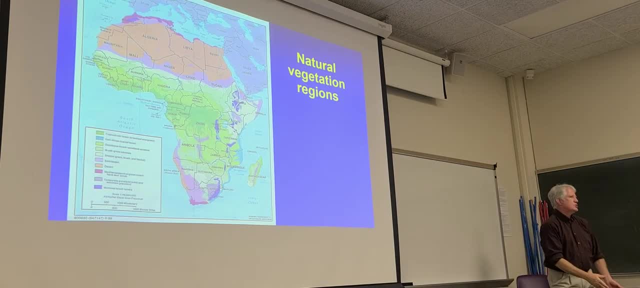 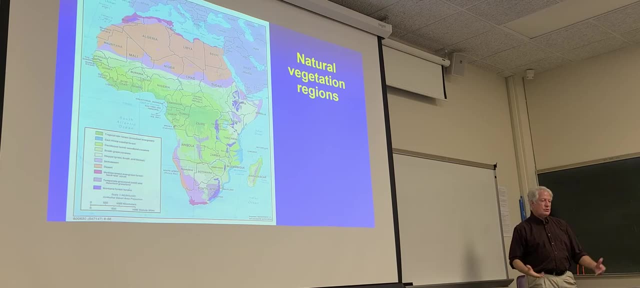 like any animal anywhere carrying capacity, they can't support huge populations. they may not have a robust economy because they don't have a port. they don't have a lot of goods on the on this to barter on the world stage, right that other people want something unique. 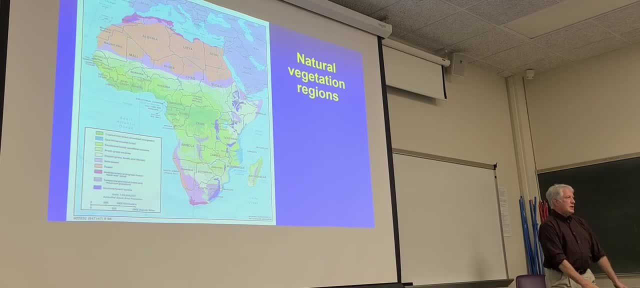 unless they have something unique right. so many of these countries don't have anything. other ones have a lot: botswana diamonds, democratic republic of the congo, rare metals, the uranium. the bombs of world war ii came from there, right, the old belgian congo gold, right otherwise. 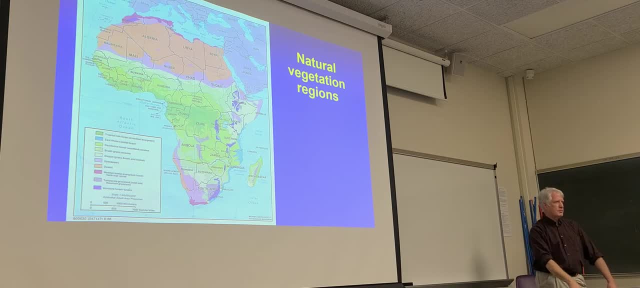 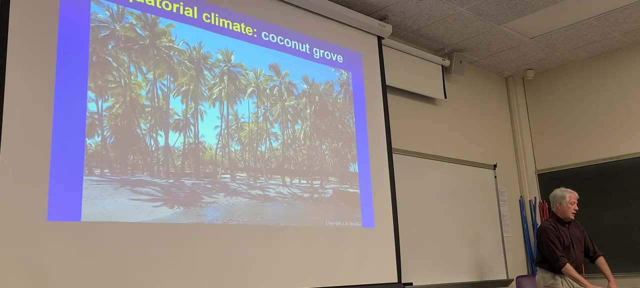 you're going to have other unique things like ivory, right out of the world market, but there's a ban on that. so it's a complicated story, but it all traces back to your geography, pulsing back this. these are just shots of different types of climates as you dry out, but this is kind. 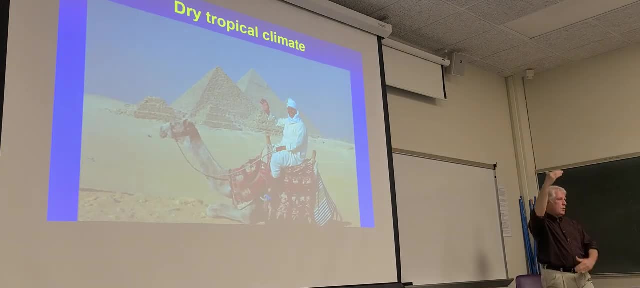 of where it started, and as you work forward, right away from the equator, you're drawing things out. why were there such a huge civilization here in egypt, though? right one, we had to know it was there. there's got to be something left behind if it was in the jungle. 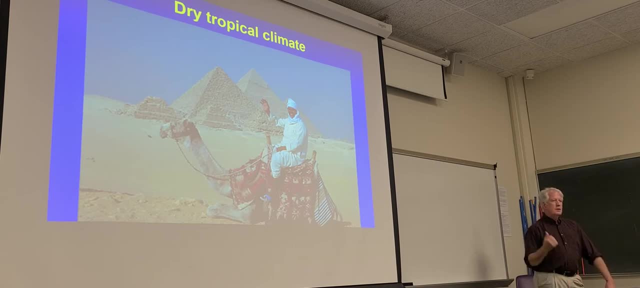 it's either going to get covered up or it's going to rot away. if it's organic, it's because it was on the nile, the nile, right. so you had a flood plain of the nile. it's like a ribbon of life, right, right. 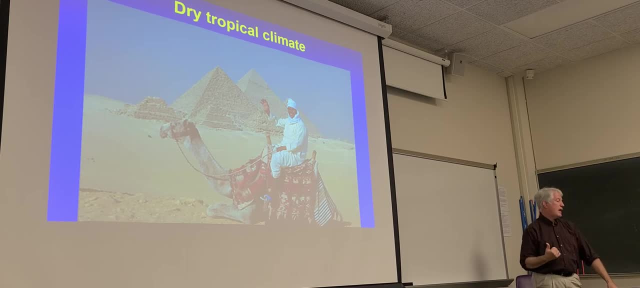 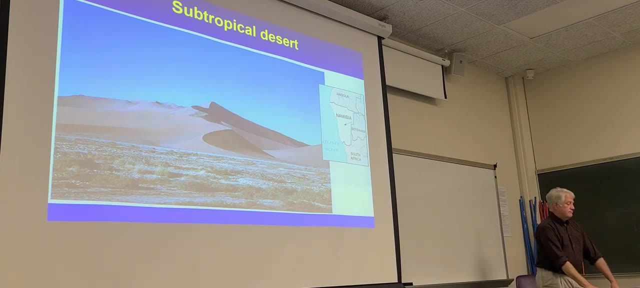 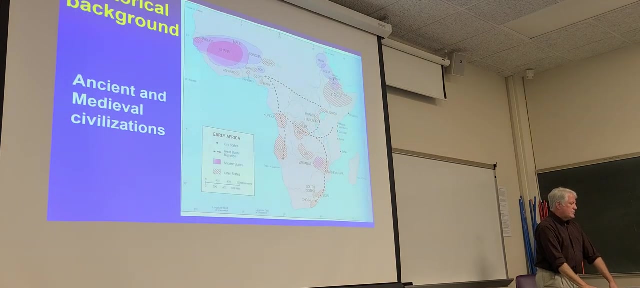 desert sands there allowed for this particular civilization to leave these remnants behind. so those are behind. many other places don't have this namibia, for example: drifting sand dunes. we either covered everything up with anything was there or never had a total historical background. we tend to think of european history. 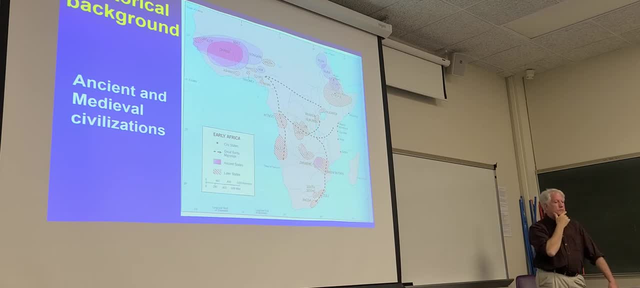 um or the mayans. but there are some great kingdoms in africa, some of which still exist even post colonial times. ghana, for example- that was the name for the country there. but other ones- the banglola balozi, the balunda, the congo baluva- are still there um great zimbabwe. 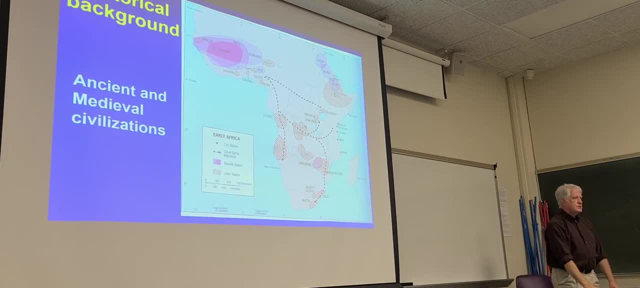 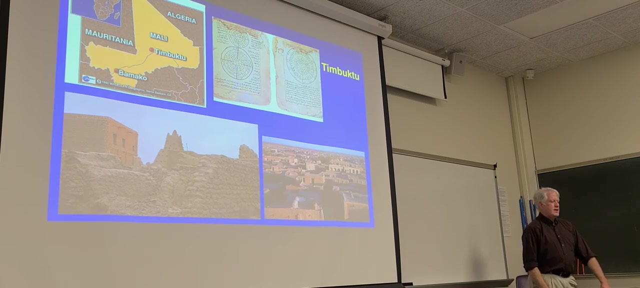 south africa, right, ethiopia, many of these are still. you know um, many of these kind of up, some cultures. one, by the way i said, remember many of these are still intact. This one: you may have heard of Timbuktu. Right now it's thought to be: wow, it's far away. 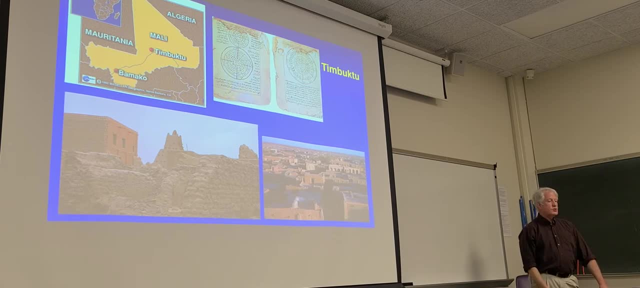 It's like man: he's off to Timbuktu. It's far away. Well, it used to be on a crossroads, a trade, and it's a site of learning. There are still families there with documents that, because it's so arid, are still. 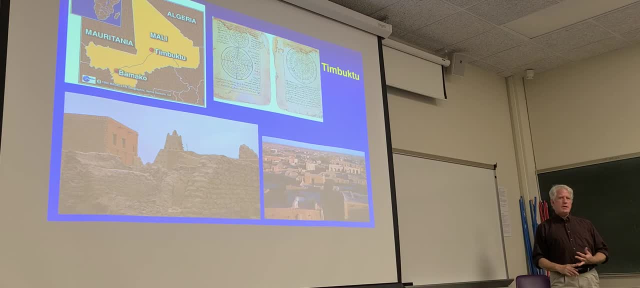 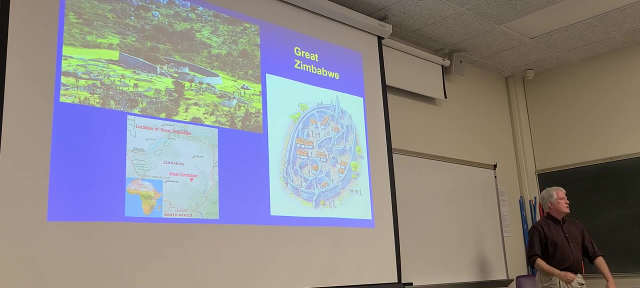 have rotted away of medicine and astronomy and quite a seed of learning there that are preserved over this time. It was a repository of knowledge here for the region. Great Zimbabwe is another example. The only reason we know this here is because some of the things, the things that rotted away, could have rotted away. 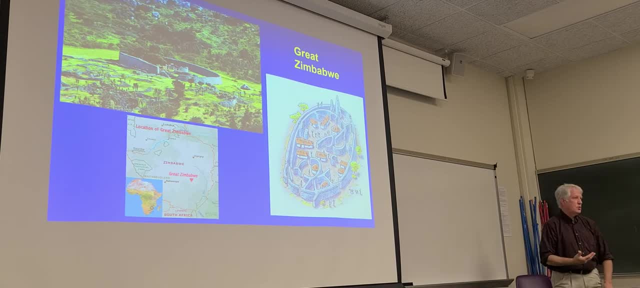 but they built some things in stone which are left behind, Kind of like the Mayas. the only reason we know the Mayan Empire was there was by some of the hard remnants that were left behind. But this was, this showed an organization that was beyond just. 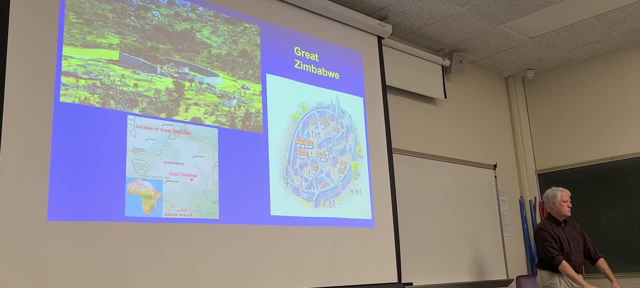 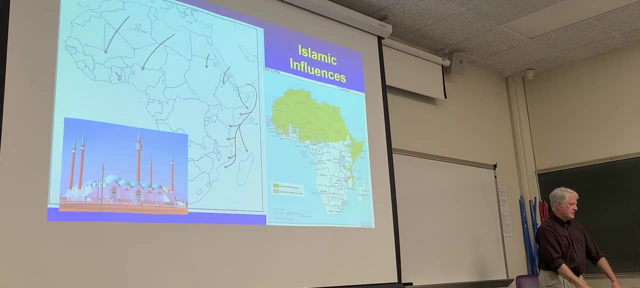 pastoral life. This was, you know, quite a good organization there. that doesn't exactly exist anymore, but we know that there was some type of organization there in the past. Now, other influences on the African from outside- right, This is the thing. 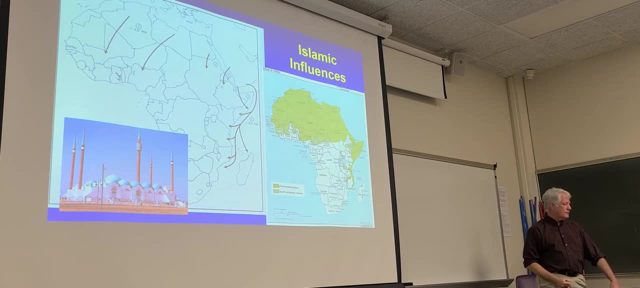 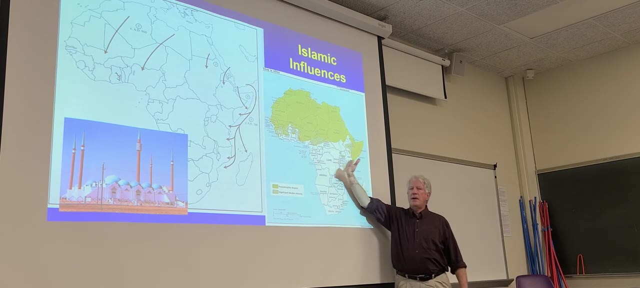 Everybody's influenced from the outside by somebody. but they had some other influences. So the Islamic influence from the north can certainly be felt and there's a certain amount of line here, because this is obviously just by trade and other things. So you know, trade from the 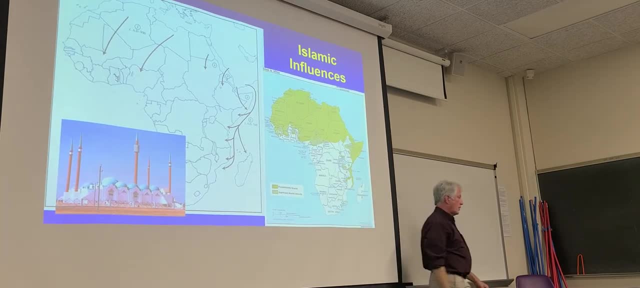 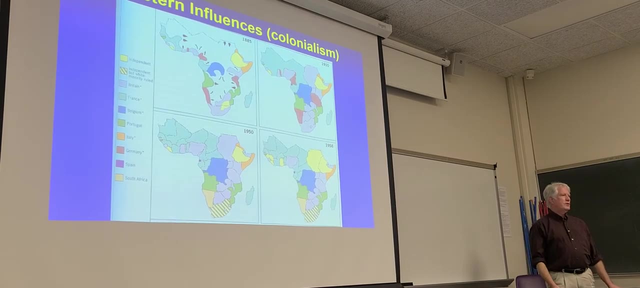 from the east and then certainly coming down from the north. There are great Islamic influences in Africa. Other influences that come to mind- nobody really mentioned- was colonialism. It was hard to get into the interior, like the old Livingston, I presume. 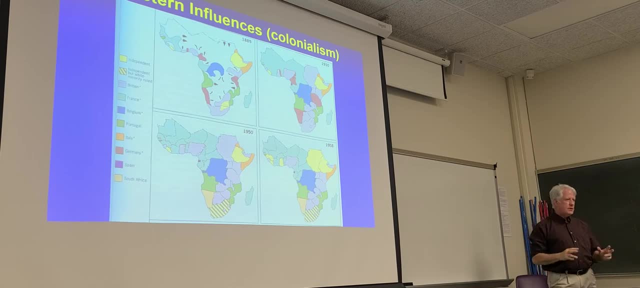 Dark, you know dark Africa. It was mainly because you couldn't get into the interior very easily. None of the rivers really went into the interior. The Congo River, which flowed right out here, right at the mouth, has a bunch of rocks. 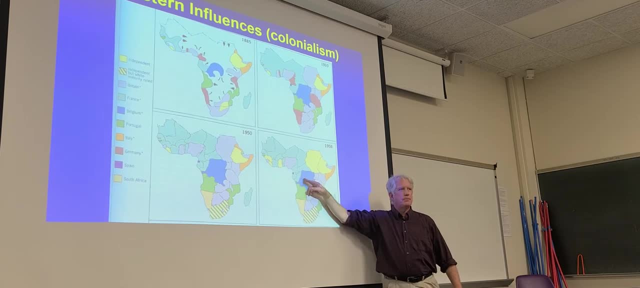 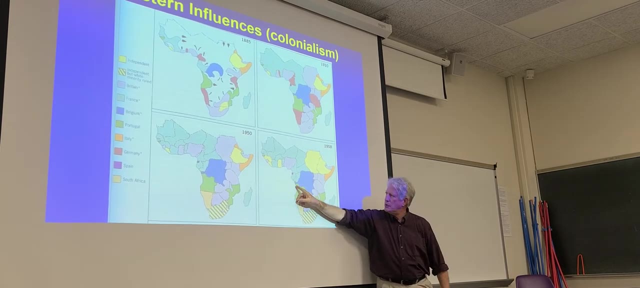 So, even though it's a good navigable river upstream right there, you couldn't bring seafaring vessels in. When the Congolese- sorry, when the Belgians- came in, they built a little railroad around it, right, so that you can come in, unload, bring it around, load it back up. 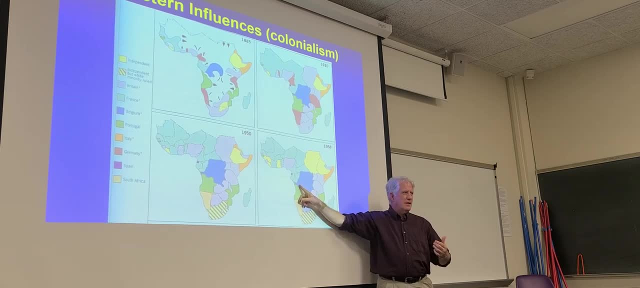 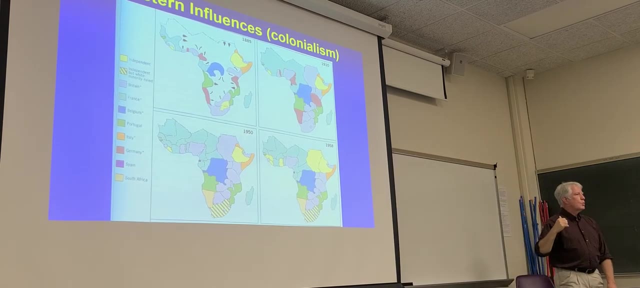 But any time you get a nick point, that's basically a hardship that you can't easily conquer. You can't easily get into the interior. So a lot of these Western influences were trying to get into the interior To get the goodies right, to get the gold, the animals, the exotic animals, the ivory right. 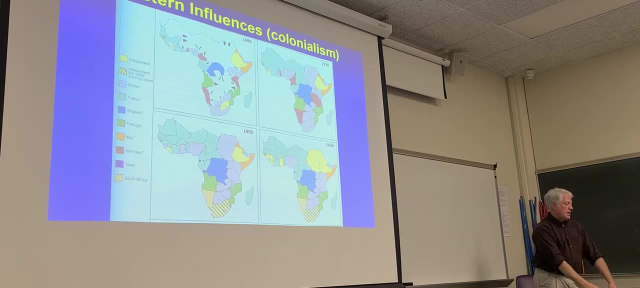 And then, certainly with slavery, the people. So this was carved up like a turtle. This was carved up And unfortunately, if you look at some of these borders, even back here, those are still the borders today And it's given them no great benefit and mostly trouble. 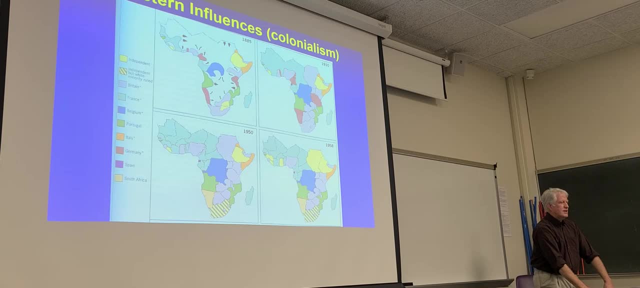 It would be much better if they all would sit down and say: you know, let's just get rid of some of these fictitious borders that colonialists left us with and get back to our normal divisions of tribes. But it hasn't happened. 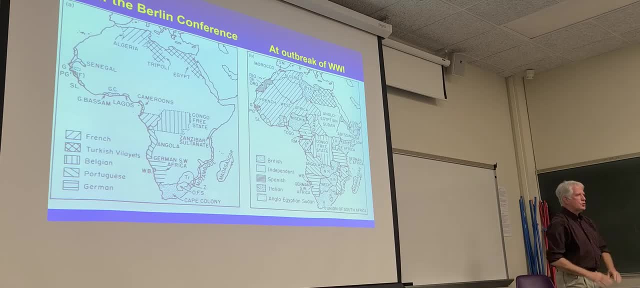 So after the Berlin Conference Congo Free State was given to the King of Belgium, The rest of it was carved up. West Africa largely went to the French, East Africa largely went to the English. Italians had a run, in some places Germans. 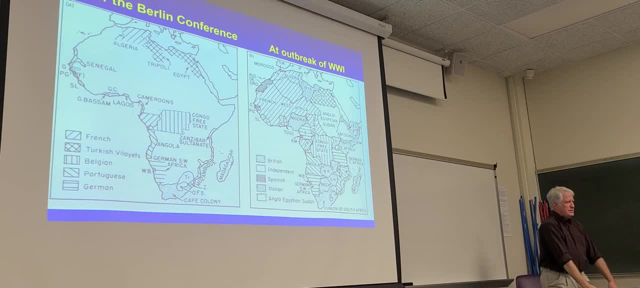 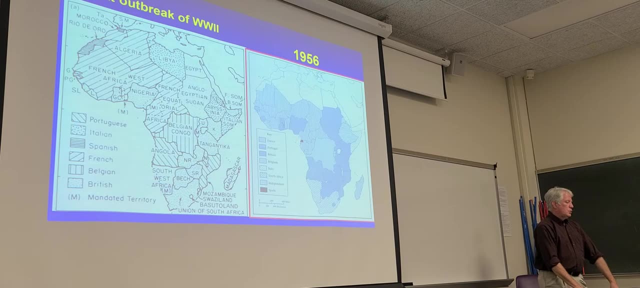 Portugal. But you know they switched hands as wars, as external wars, happened. Then you get up to outbreak of World War II. here There's the Belgian Congo. This looks a lot like some of the current borders of some of these countries. 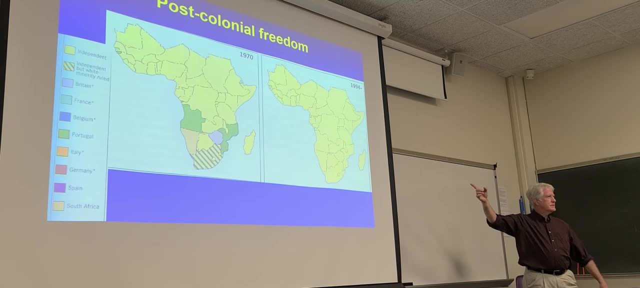 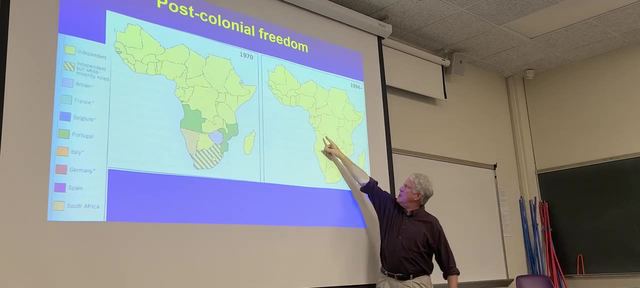 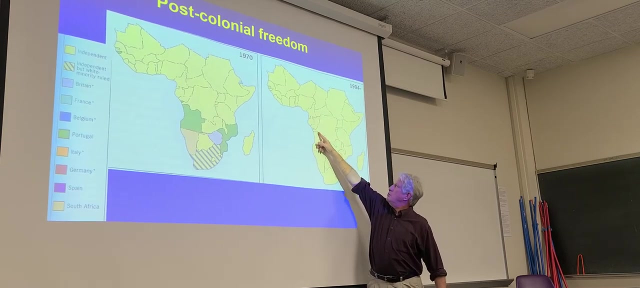 Post-colonial. now we have this right. So why do I say this is problematic? I was stationed a couple years right about here, Right, Very close to the Angolan border, In the same tribe. the Bachoque were all in this region here. 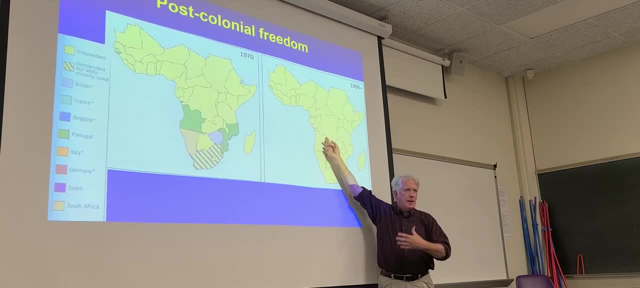 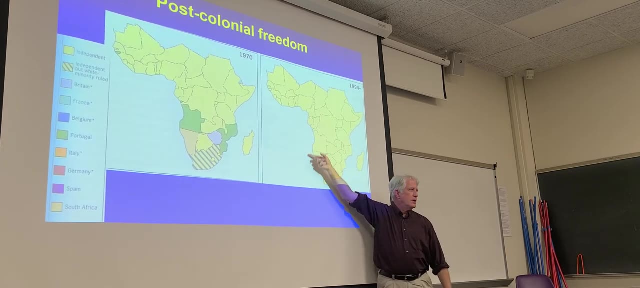 and they would cross the border because they were all family, right? But technically, Angola was a Portuguese-speaking country and this was Belgium, so it was a French-speaking country. So the official languages were different, right? But that didn't matter because they all spoke Pichoco. 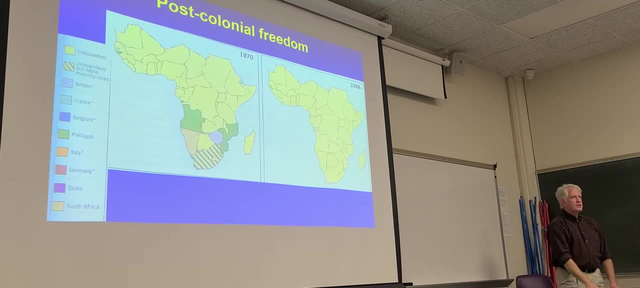 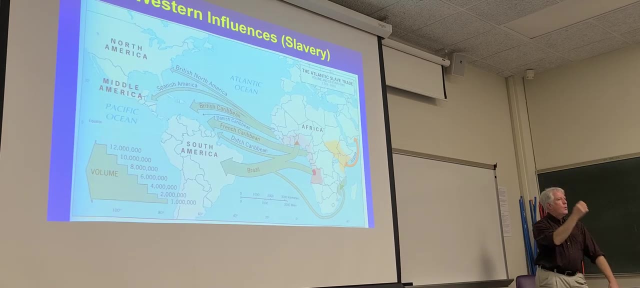 But they forcefully went across the borders. It wouldn't have mattered if you just kind of said, let's keep the tribes together and re-divide this, But that didn't happen. One of the other influences on Africa from the outside was obviously the slave trade. So much of this went out towards West Africa. Why this particular pattern? You can take a whole course on this. Remember this was the days of sailing ships and not self-powered ships. They had to have a tailwind, So generally around the equator, not right on the equator. 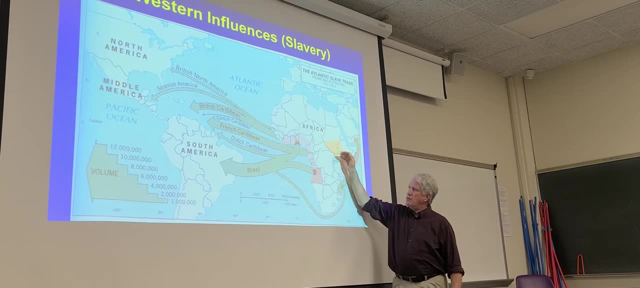 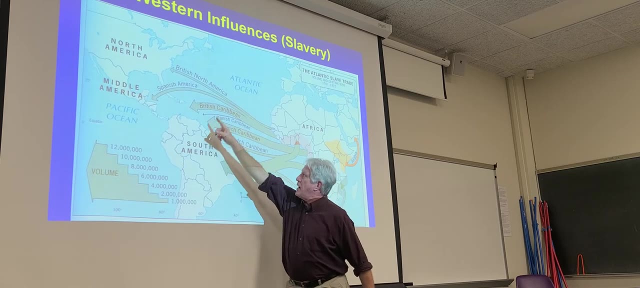 but just scoochy to the side of the equator. here you have winds that blow from the east to the west. So think about this pattern, right, This clockwise pattern in North Atlantic. You catch a tailwind. It blows you over to your plantations here. 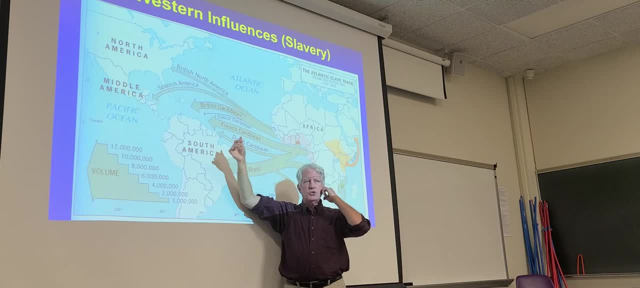 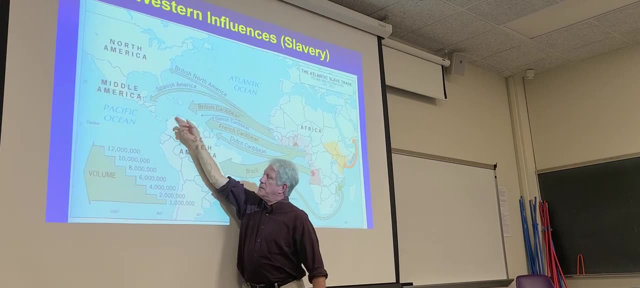 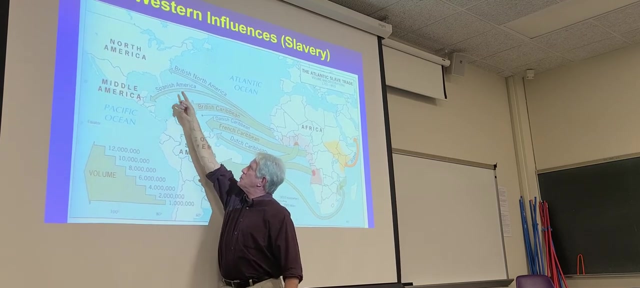 where you can unload slaves to work it, because that work is hard and all the people from Europe don't want to do it right. Gather together whatever's there: the gold, the cinnamon, the pepper, whatever it might be, tack your way up the coast. 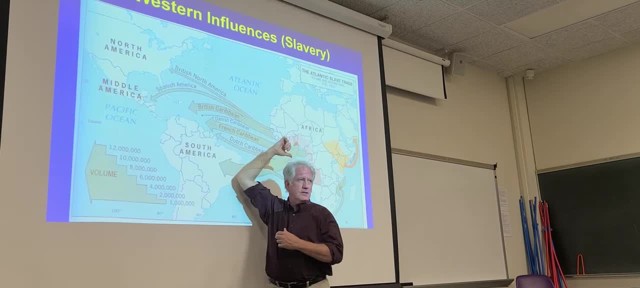 to catch the tailwinds going from west to east, right. So where does our weather come from here? It comes from the Dakotas, from the west. You want to get that as your tailwind to blow you back and your journey's complete. 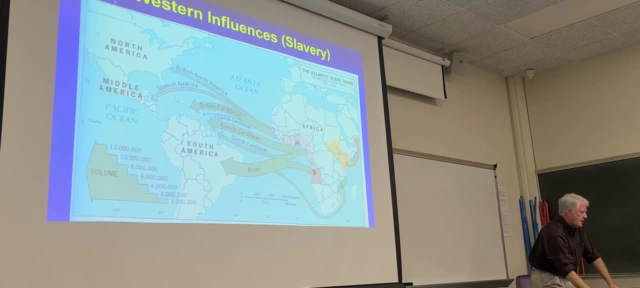 You make that big circle. Where are there a lot of shipwrecks at this time? That tack trying to catch go from the tailwind from the east to the tailwind from the west going up the coast here. So you have this as the primary slave trade. 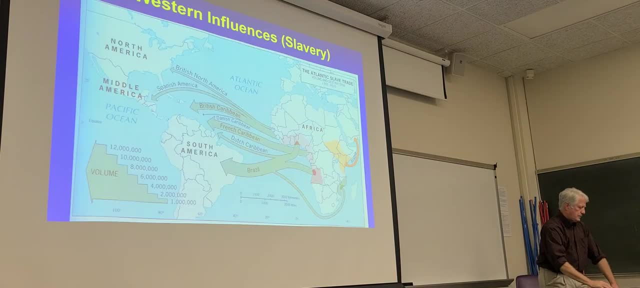 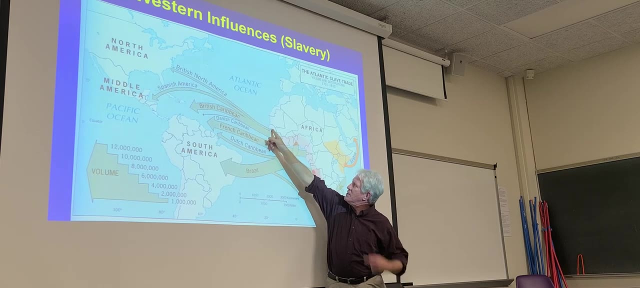 Gorian Islands, West Africa. This is Senegal. It's the westernmost point in Africa. There's the nose. It looks kind of like a lion here. That's the gambia that sticks into it like a finger. But off this shore, here is Gorian Islands. 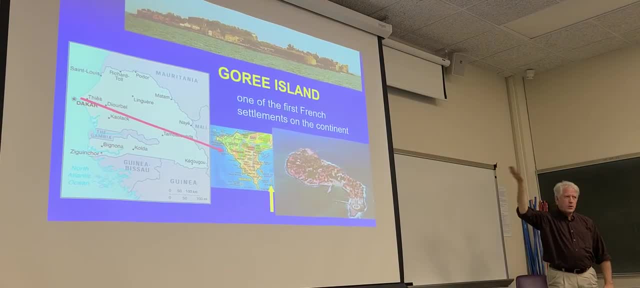 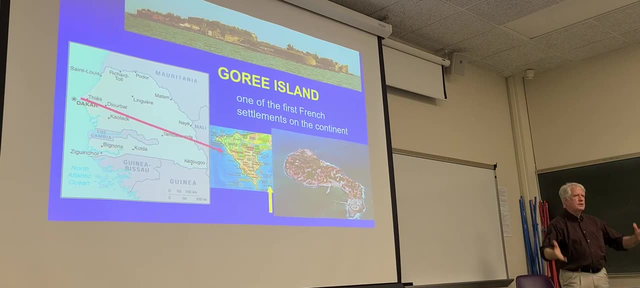 world heritage site right now. But that was an island And look, it's a fort, It's fortification. Slaves were property and they were expensive, So you brought them in there and you held them until a boat came up to buy them. 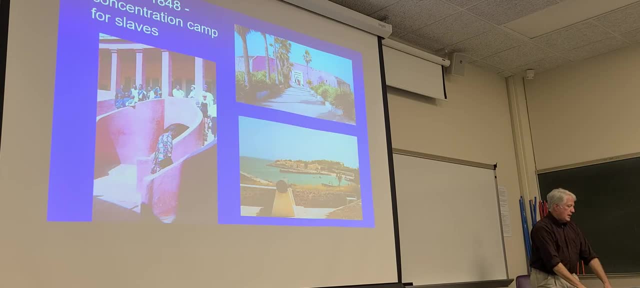 So a fort was there to protect your asset, And this was the slave trade house. Slaves were kept up top in back rooms, marched down these two staircases And that image on the left Sold in the central courtyard And then out this door. 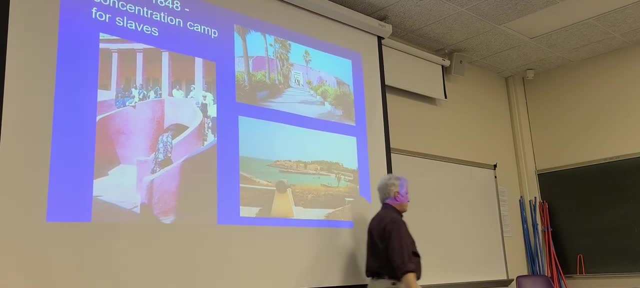 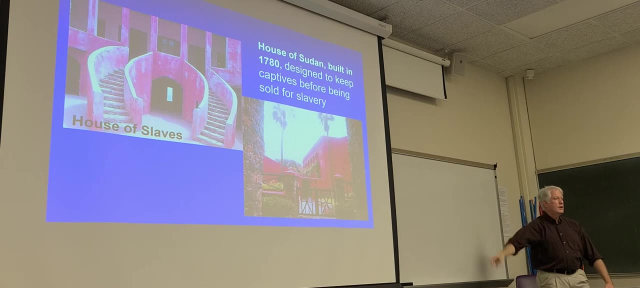 There's a door here. I think I'm going to have another shot of it. They would put a plank. Yeah, there it is The door of no return. So you went out that little door after you're sold onto a plank and you're off to you know. 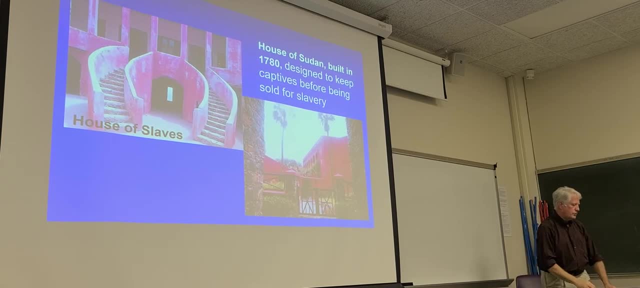 the west. You're off to the quote unquote- new world. This is some shots that I took when I lived there. So Gorian Islands is now a world heritage site. You can tour this, But this was there for quite, I mean hundreds. 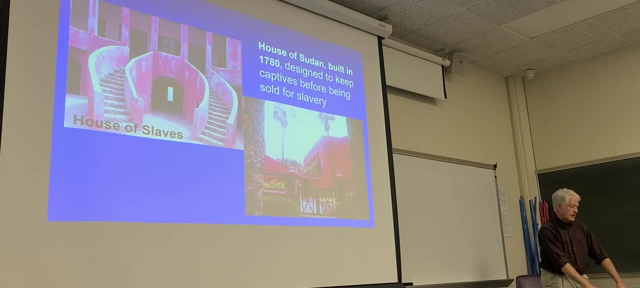 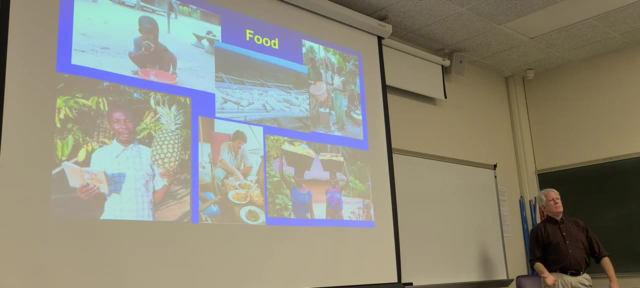 I mean, this is a long-term investment here on Gorian Islands off Senegal, So all slaves are brought in from all parts here to be sold and then off they went. Food- Everybody else think about food. How many people are in the world right now? 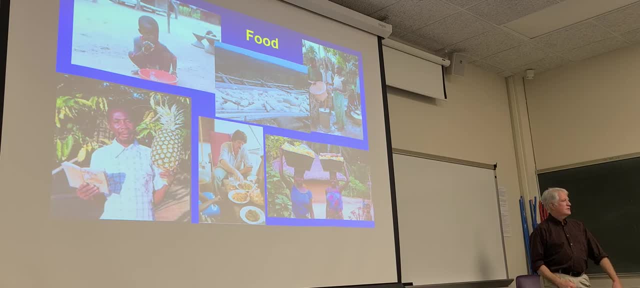 What's the world population? How many? Yeah, a little more than north of 7 billion. I was born in 1958 and there were a little over 3 billion people, So right now, probably before some of you graduate- it's going to hit 8 billion. 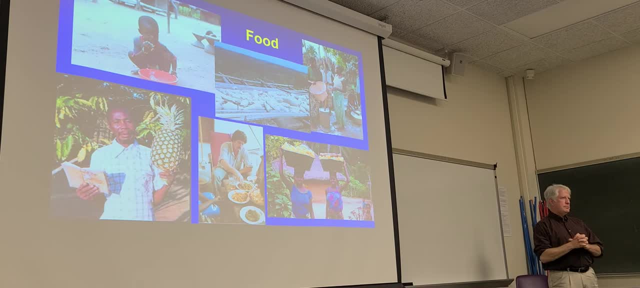 So 8 billion people 2050,, 9 billion 2100, so the end of the century, 11 billion people. So when it always comes back to how you're going to clothe, feed, et cetera, 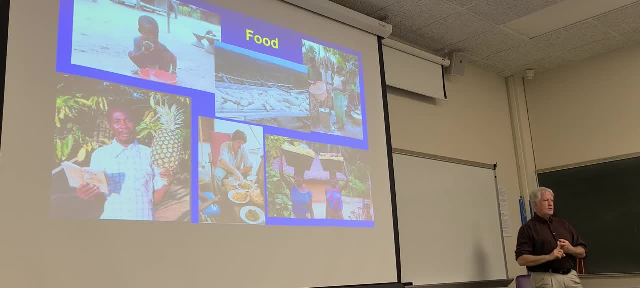 especially the feed, because you know we need to breathe, you know about every couple of seconds We need to drink, but we need to eat every day. It's not like you can say: you know we'll eat next week, right. 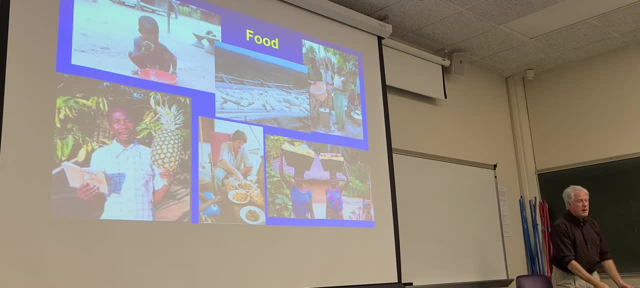 No, we need to eat every day. So with every one of these bodies comes two hands to work, yes, but also a mouth to feed, And that's a struggle. It's getting better, But that's a struggle. That's still a struggle. 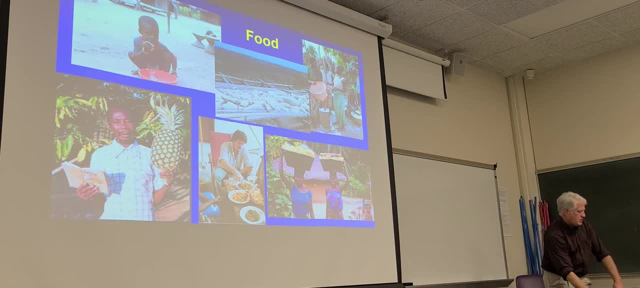 These are some foods. I'll just go through some foods. This is me back when I had a cheesy mustache chowing down, And this was in Zaire. It was very communal eating, Kind of like if you go to an Ethiopian restaurant now. 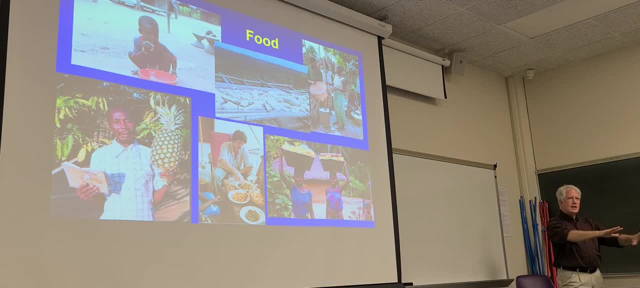 you get couscous or something or flatbread and you always kind of sit around and pinch it off and eat it. Yeah, very communal, right Same thing there. So you have different foods, You all sit around and eat communally. 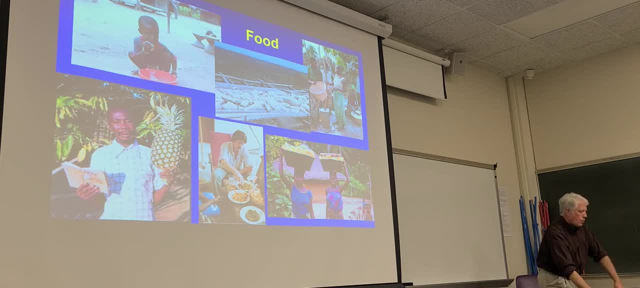 Nobody has their own plate. You all just kind of share it. So, whatever, basically they can grow One of the in some areas. in this particular area, protein was a little bit scarce, so you might be eating some non-Western diet protein sources. 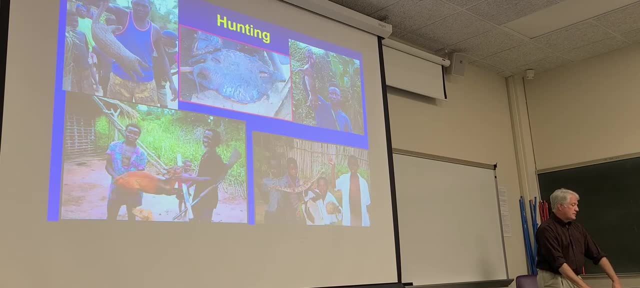 let me put it that way. But a lot of things could grow right. So hunting was a big thing, Not for big animals. Those were mostly hunted out like elephants. Sometimes they get a hippo Dig, dig, dig. 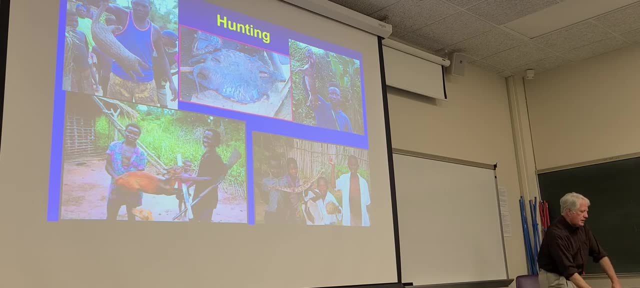 Dig, dig or an antelope, et cetera. But you know, cat rat that's a pangolin or a spiny ant, eater, Snakes, birds, bats, rats, cats, Any pig, Anything. In Zaire, everything but frog legs. They wouldn't eat frogs because they thought it would make you go sterile, So frogs were off the table, But almost everything else would end up in the stew pot Right. This is from Senegal, West Africa. Fishing is a big one. If you go to the coast, there's a good source of protein: What isn't bought at the beach, What isn't bought at the fish market that day. It's usually dried and then shipped to the interior. 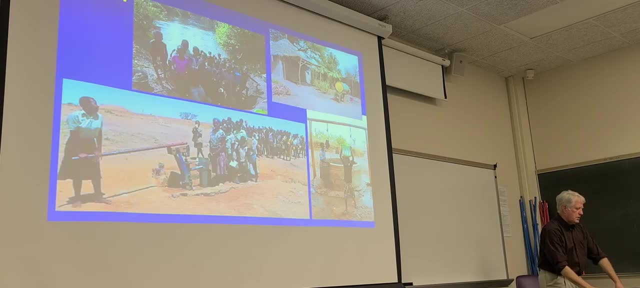 or exchanged for things in the interior. So it's a great barter system. back and forth Water Again: if you have surface water, that's great. If you don't, it's well water. So this was a shop in Senegal. Hand dug very deep. well, as you can imagine, These kids have to go out, sometimes a couple of times a day, to pull enough water for the family because, with no rainfall replenishing it, they've got to wait for more of that ancient groundwater. 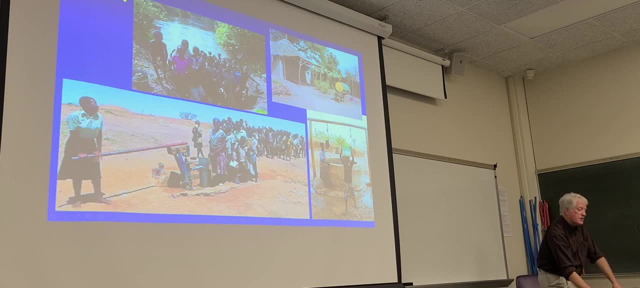 to kind of seep in there, Right. So this would be this, which is a lot more protected from disease or something getting into it. But if you're in surface water generally, you'd pick a spot where people wouldn't bathe. 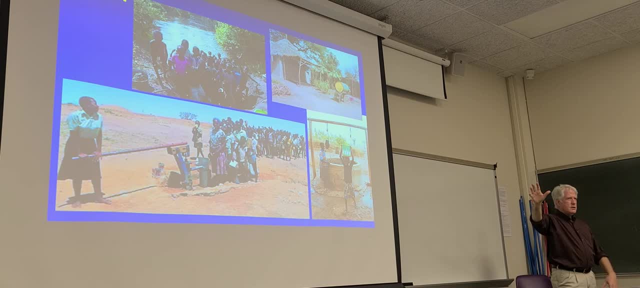 So if a stream comes in, you would say: you're drinking water here, women bathe here, men bathe here, Right, And you have that division there that keeps your water source very clean. Challenges: Some challenges. These aren't unique to Africa. 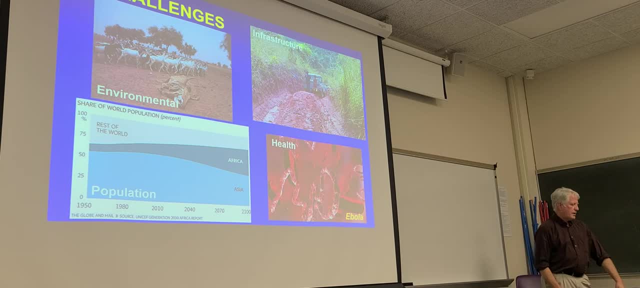 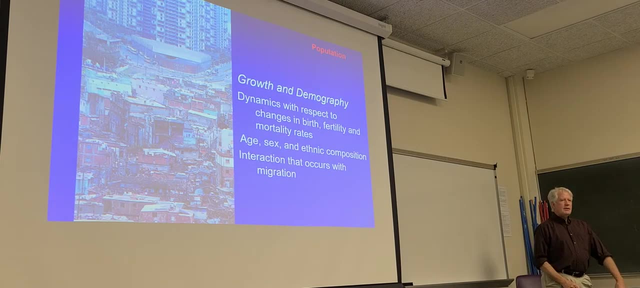 but they seem to be not being resolved all that quickly there: Environmental infrastructure, population and health. So let's take them one at a time. Population: Even in the United States, how many of you are going to go back to being on a farm? Probably very few. The goodies are in the cities, right. That's where the nice stuff is, That's where the schools and hospitals and sports and movies and food and dynamics are right, Not out in the rural areas. Same thing here. 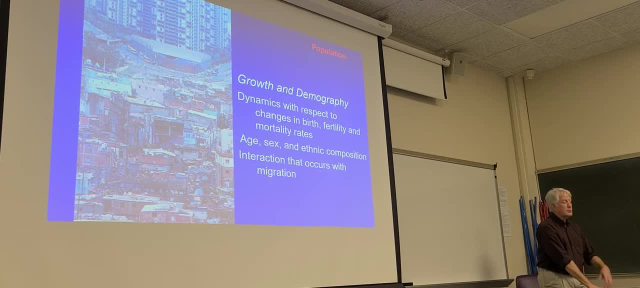 People don't want to be in the rural areas that much anymore. They're going towards cities for the promise of a good life. But some of these cities you can see were never designed or meant to hold that many people. Cairo is groaning under the weight of the people. 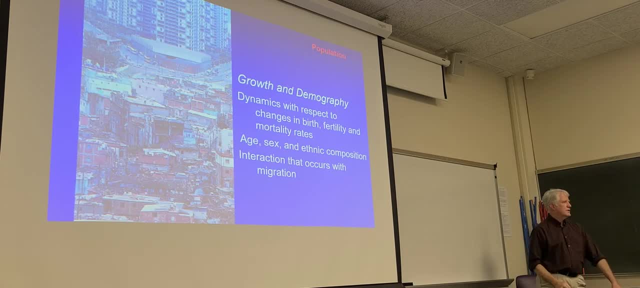 that are trying to go to Cairo, as is Mexico City, right Some of these areas, the city is the salvation, especially perhaps with climate change. We have some climate refugees, but growing populations and moving populations is the name of the game, right. 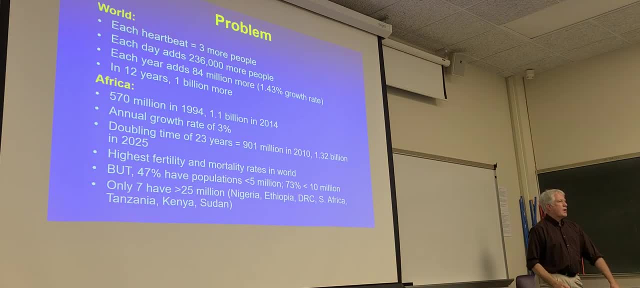 Not just in Africa, but around the world. So this is the problem. We're about almost 8 billion people now. They're not equally distributed around the planet, and certainly not equally distributed in any one country. Some of the highest fertility rates are still in Africa. 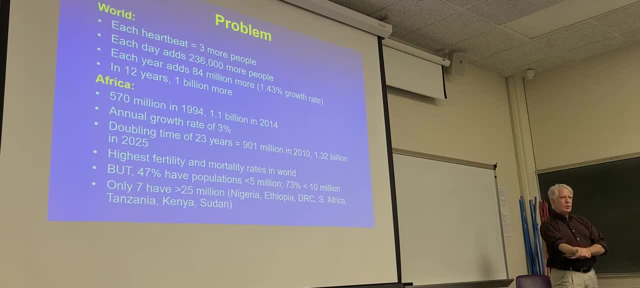 Some countries are shrinking- Poland, Italy, Russia- they're just not there. aren't enough Italians making more Italians right? Their population is growing. There are more people dying than being born that are Italian. Some other countries: there are more people being born than are dying. 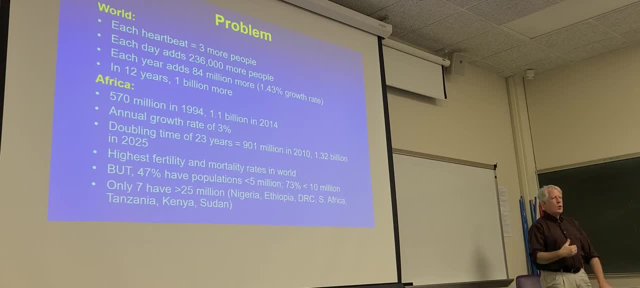 And that's not a bad story, right? We don't want infant mortality to be the limiting factor on a population growth. That's a tragedy. So you have to look at the women. How many babies does a woman have in her lifetime? 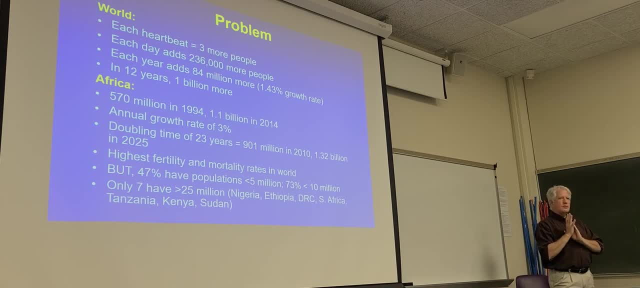 Men don't count, It's the total fertility rates, It's the number of children that are being born. In my family I've got two kids, a boy and a girl. So when my wife and I die, the two kids take our place. 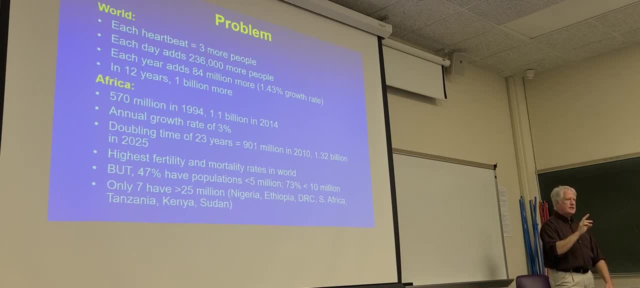 and there's zero population growth. If you have more than two kids and they survive, you have augmented the population, all right. If you only have one kid, you decrease the population And it seems like through garrative factors that Africa still hasn't quite got a handle. 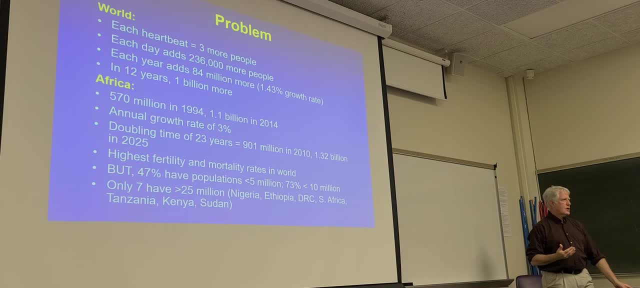 on its total population growth. Some of these are in their control and some of them aren't. For example, you don't have to worry about Social Security anymore. There's Social Security, So even if you're destitute, there are things that'll take care of you. In many countries again, not just in Africa- your kids are your Social Security. If you don't have kids, who's gonna take care of you at your old age if the government can't? So you're gonna make sure you have kids. If there's a high infer mortality rate, you're gonna make sure you have more kids, because you can count on a couple of them dying and you want at least some of them to survive and make it to take care of you when you get old, right? Plus, if you're more agrarian, many hands make light work and on the farm you need to work right And to pay for it you need family. So all of this- it's not unique there, but it seems like some of the highest fertility rates. 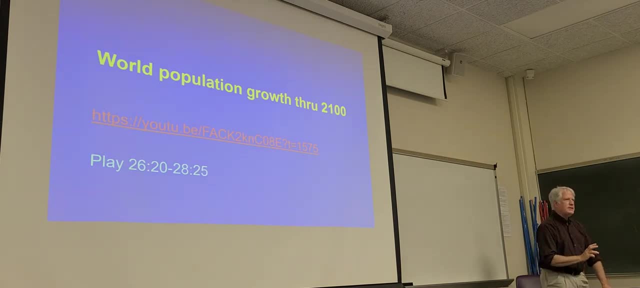 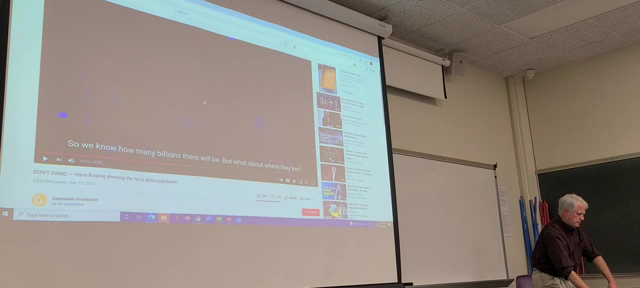 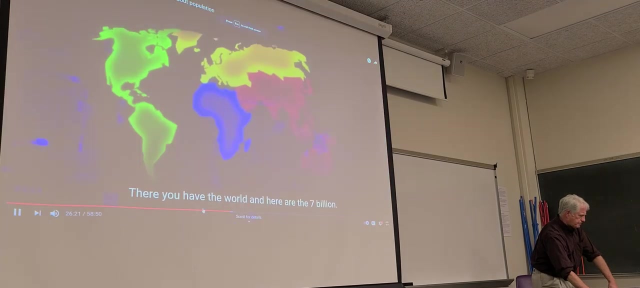 are in Africa. I'm gonna play this quick video clip and it'll explain this a little bit more about not where we are now, but where we're going and why Africa seems to be having some more challenges than other developing countries. There you have the world. 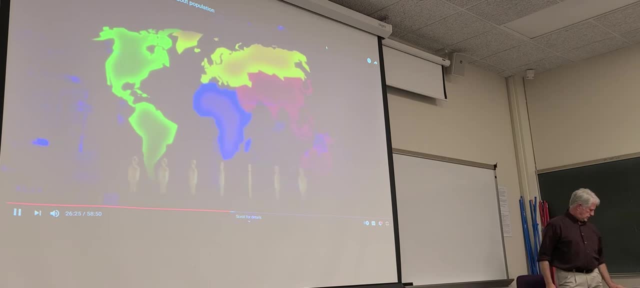 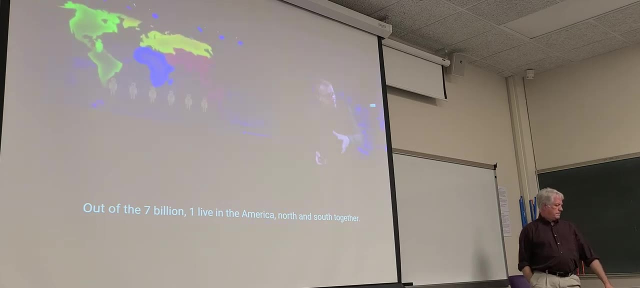 and here are the seven buildings. Now, out of the seven buildings, one live in the America, north and south, again One in Europe, one in Africa and four in Asia. So this is now but how to remember this. I have a very simple way of remembering this. 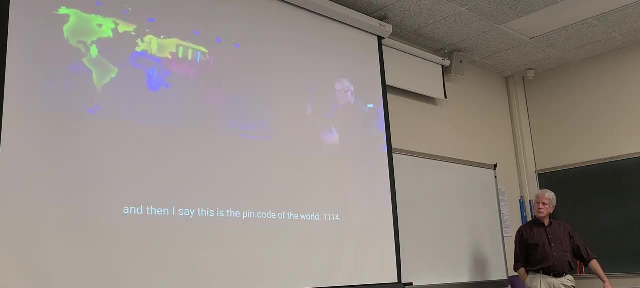 I put up the numbers like this and then I say: this is the pin code of the world: 1114.. Now what will happen up to mid-century? That will go very well. Europe: no increase. In fact, the European population has decreased. 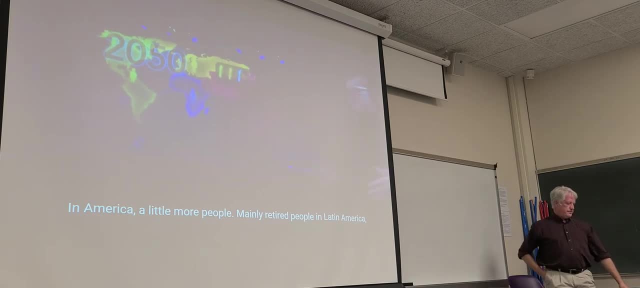 In America a little more people, mainly retired people in Latin America. so it makes no difference, It's more or less the same. In Asia we will have one billion more, and then the population growth in Asia, In Africa, in the next 40 years. 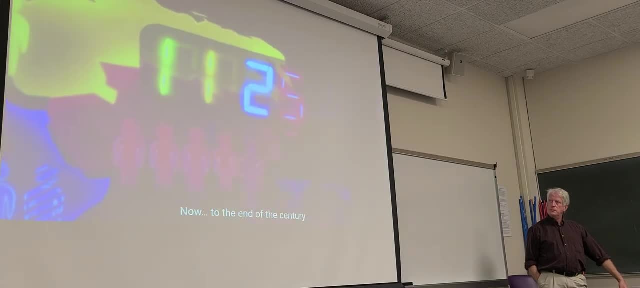 the population will double for two years Now, to the end of the century. Well, we know quite well. no more people in Europe, no more in America, no more in Asia. but Africa is set. as we have data today, 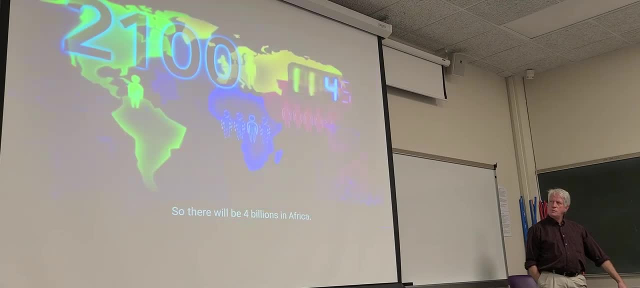 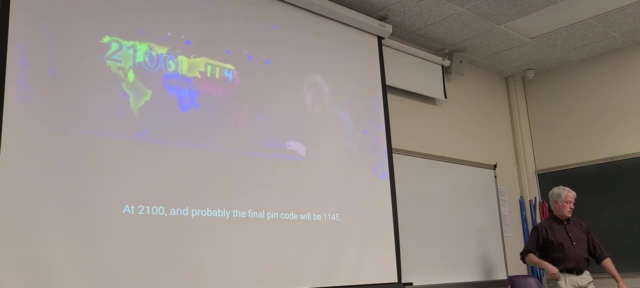 for another double. So there will be four billion in Africa, The 2100, and probably the final pin code will be 1145.. So in 2100, there will be quite a different world, The people who live in what I call the Old West. 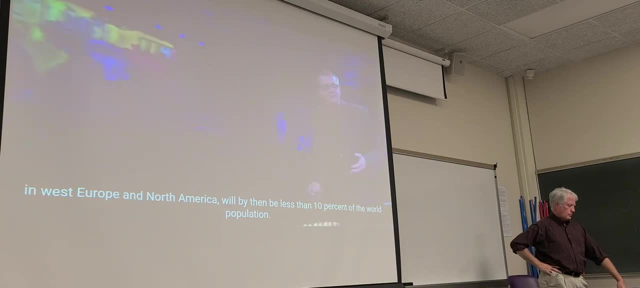 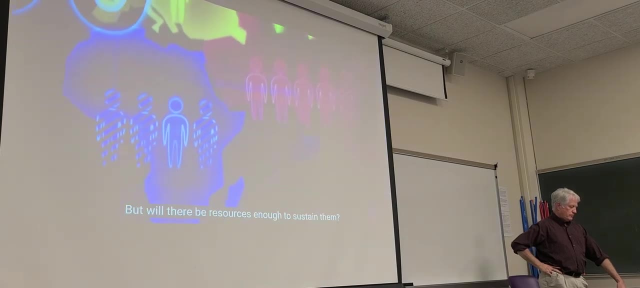 in West Europe and North America will, by then, be less than 10% of the world population. 80% of the world population will be living in Asia and Africa. But will there be resources enough to sustain them? Well, this will be a huge challenge. 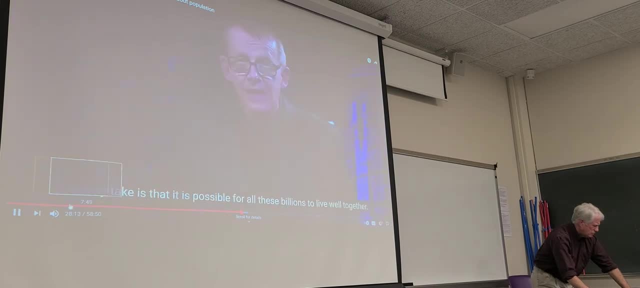 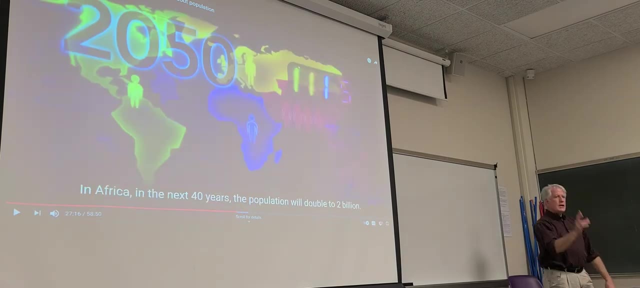 and nothing will come automatically. Mike, Let me pop back to this here. All right, China. You may have heard One child. Yeah, Why do they? why does he think that the Americans aren't going to grow up? So what's the reason? Because our populations are already shrinking as it is now. We haven't grown. Africa, for example, between the 94 and 2014, doubled its population in 20 years, Whereas we, even in the United States, we're shrinking. How are we going to fill that gap? 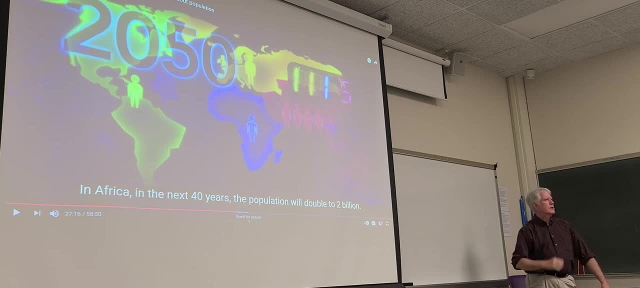 How is Italy filling that gap? by immigration. But then the people come in and say: they don't look like us, They're not Italian, They don't have the same, They don't have the same food or dress or language or religion. 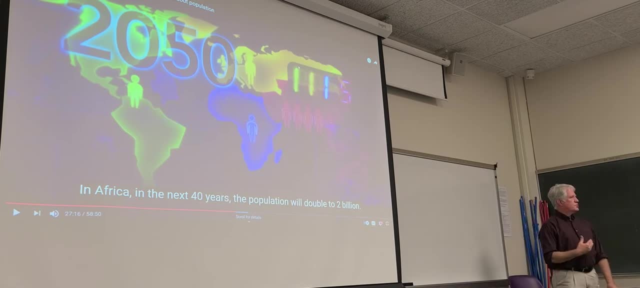 I mean there's going to be conflict, a little friction there. that's going to happen. But as far as overall population first, we've already hit two billion children. There are two billion children in the world, and that hasn't changed. 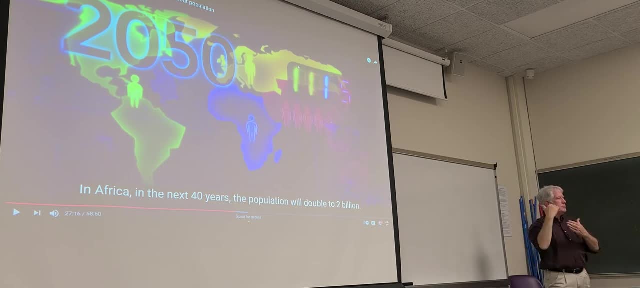 for many decades. So they postulate that that's not going to change. We're going to hit 11 billion by the end of the century, just by as those two billion grow older and they have two billion kids of their own- an inevitable fill-up of adults, right? 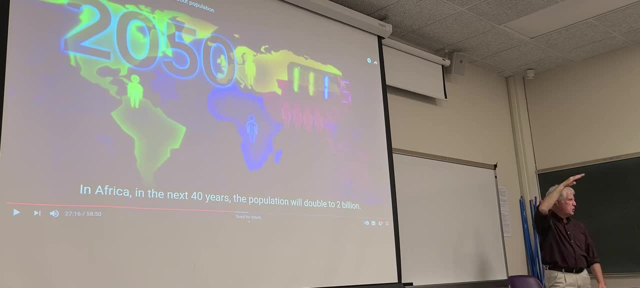 We're also living longer, so there's going to be a top block there of about a billion of older people. North and South America really aren't growing, as is Asia. Think about China or Asia in general, If you drew a circle right around here. 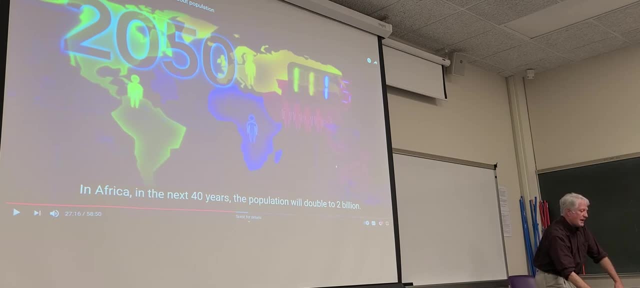 that's about half the population of the world right now that lives within that circle. They must be doing something right because they're generally being able to feed their people. You know the Green Revolution and you know rice in India or whatever. 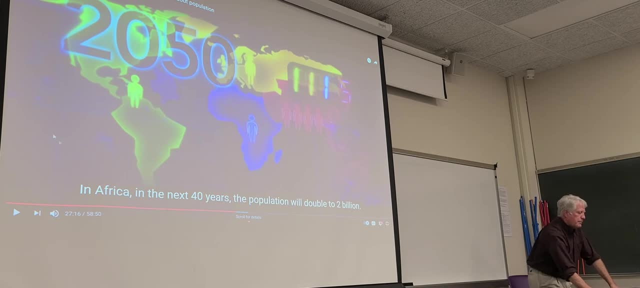 But China put on one child, one family policy. They took that away. Recently they took it away and said: you know, we're going to have two billion children instead of up to three children. They're worried about getting old before they get rich. They still have a lot of pensions to pay for old people and they don't have enough young kids because of that policy to take care of the old people. So they want them to have more kids, even though the population is blossoming, But it's not going. 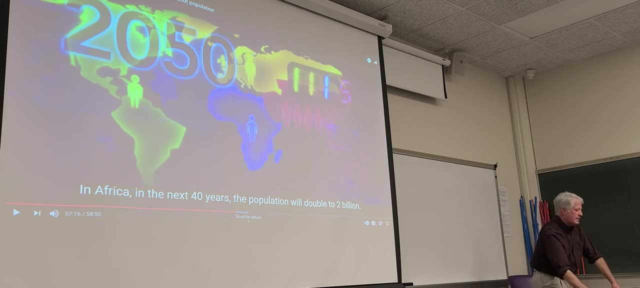 to grow that much India is probably going to surpass. But their population is coming down. But it's going from one to four by the end of the century in Africa right now and you hear some challenges in Africa, which is one billion there, triple that. 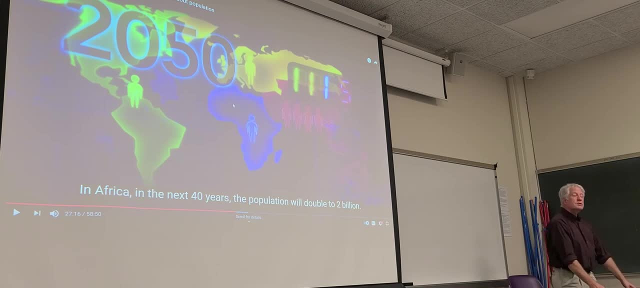 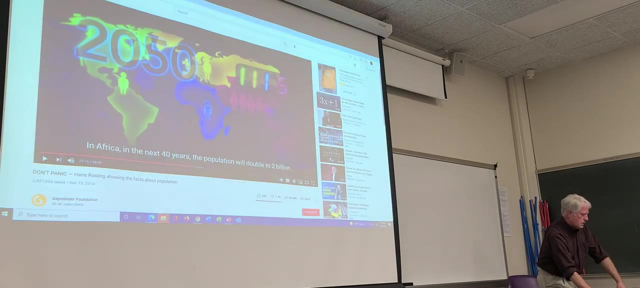 I think this is where the UN is really worried, more about Africa, sub-Saharan Africa, than it is about other parts of the world being able to meet the basic needs of their people. So, going back to some of these regional densities, Some are big countries. 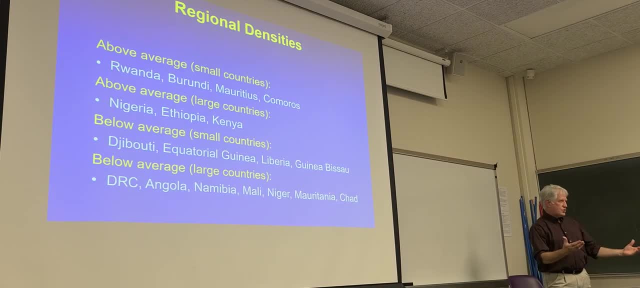 with not a lot of people in them. Right, That's just geography and that's just how regions are divided. But look at Burundi and Rwanda: High population densities, Two little landlocked countries, and the ruins are in mountains. Right, You plant a. 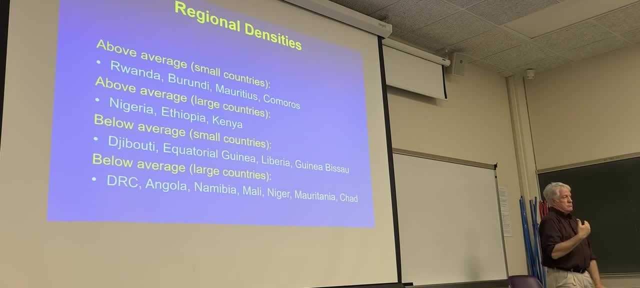 walking stick and it can grow there. They have great potential for growth Right And really just There's very similar dialects of Rwanda and Burundi, But we all know with 93, 94, the Rwandan genocide which also spilled over. 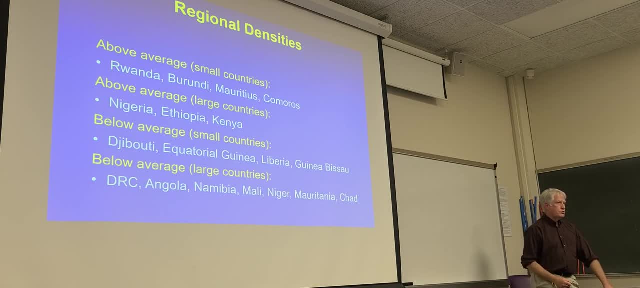 into Burundi as well as the Asian pressures and old. Yeah, There's a movie about the Rwandan genocide in Hotel Rwanda. Have you seen that? No, It was with Professor Floyd. What's the name of the movie? Hotel Rwanda? 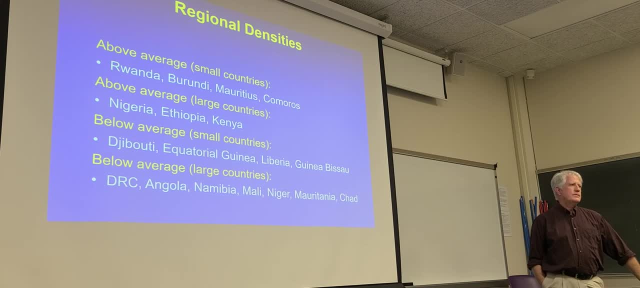 Oh yeah, That's been out for a while. Yeah, No, I haven't seen it. actually I was in Burundi. A side note: I lived in Burundi just before this. I was a student trying to protect chimpanzees and 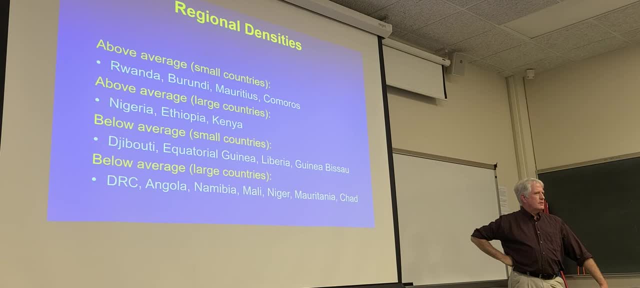 I had come from Zaire where, if you, if somebody saw you, and of course I stuck out like a sore thumb. I'm a white guy, right, I've been in villages where I've never seen a white people before. Little kids would come up to me. 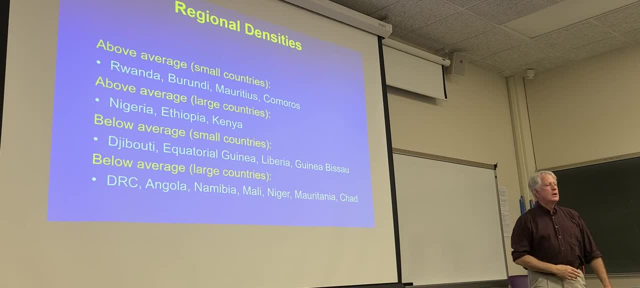 and shake my hand and look at it to see if any of the white came off. They've touched my hair and I've never seen straight hair before. I've had babies run into the run away. you know they weren't sure what you were. And others have run up to you and invite you in to eat. As soon as somebody invites you in to eat, the next one wanted to, the next one wanted to. after a while you would like, purposely like, if you had to get somewhere like go around villages. 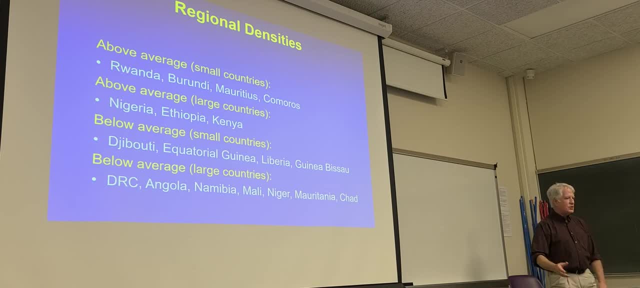 because you would never get anywhere. you wanted to go By the end of the day. you know it would be hours later. you were stuffed full, very hospitable. Senegal was the same way. Tehran was hospitable to strangers. And then I get over to Burundi. 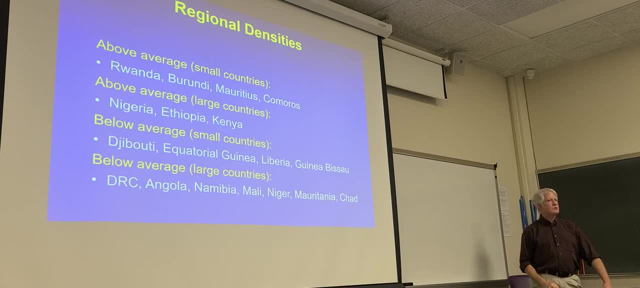 and in my six months there I never saw the inside of Burundi's house. I was never invited over. It was before you went, before I was even allowed into the country. they wanted a police report from my hometown, which I hadn't lived in in like 20 years. 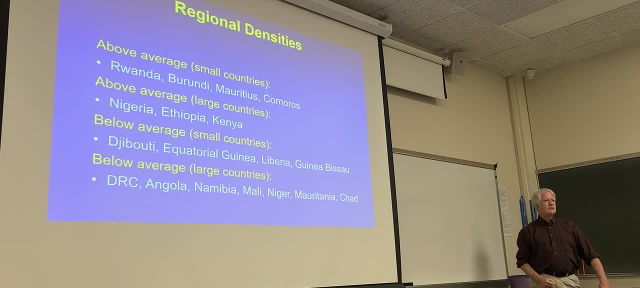 to say that I wasn't a criminal. They were very skeptical, very skeptical of outsiders right. Another one was not so much. he kind of knew something was brewing, some tension was there, Yeah, please. so here's the thing when I kind of touch on everything. 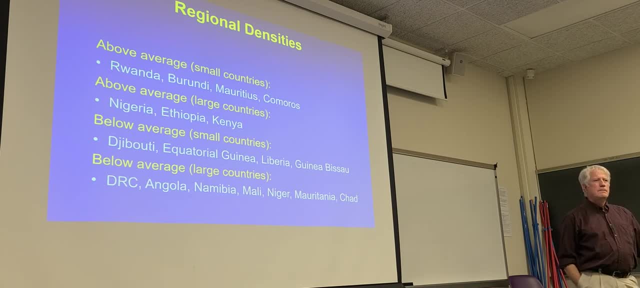 they were talking about At this point. a lot of different Africans, a lot of African countries, realized exactly what happened after the gunfire revolution and how it affected them on the long term. So now, one of the things that you have in a lot of countries, they are: 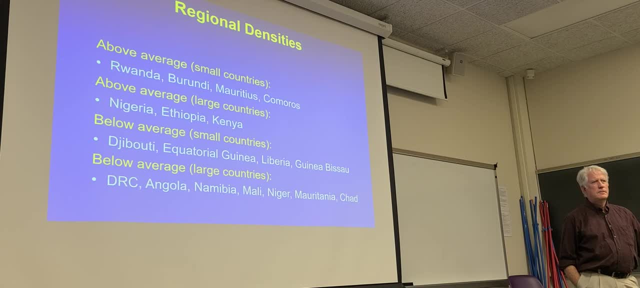 literally they. I would say it's an animosity towards Europeans. so what you said in Burundi 20 years ago, 30 years ago, that's only gotten much, much worse than some other countries and in a sense you can't really blame them, because everything that happened 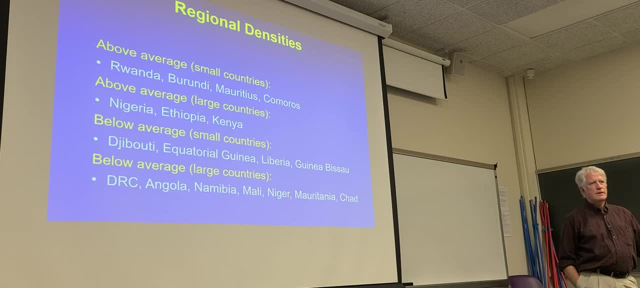 happened the way we did and, to this point, most of the wars that are happening within Africa- just within East Africa, as you mentioned Burundi- are basically colonial powers putting someone above a government in power. So kind of looking at that and you're talking about the next. 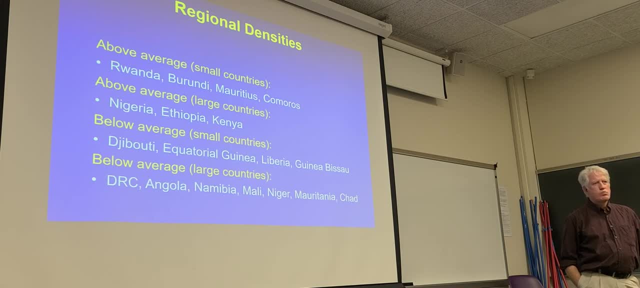 20 years, 30 years, 40 years. I wanted to ask a question to you: what do you think is going to happen within the next near future or within the next, let's say, 2050?? Well, this is this is my view, This is. 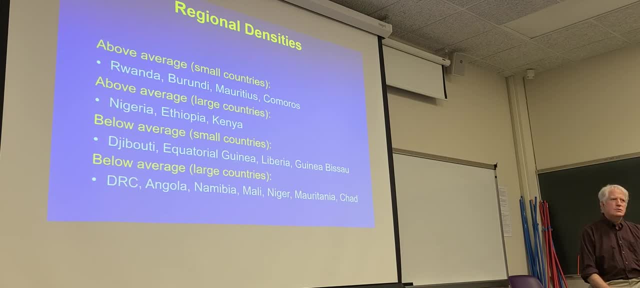 what's going on? for a while When I was in Zaire, it was the president- was Mamutu Sesese Kukukubenda Wasabanga. right, He was put in. he was a lieutenant in Belgium. when the Belgians left, there was. 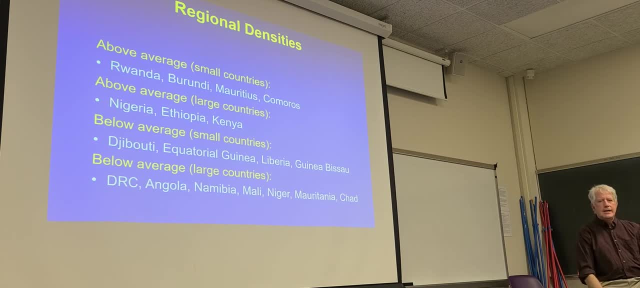 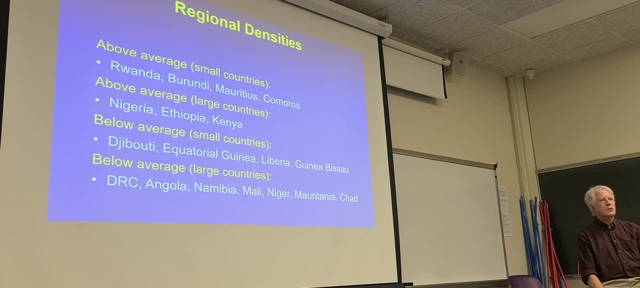 they have been the grass for a long time. i think that that i hope that that is over, that as we distance ourselves from colonialism, as we distance ourselves from the cold war, that cold war and more globalization, more information, more literacy, better health, better infrastructure, transportation, better opportunities, that to be a little bit less. 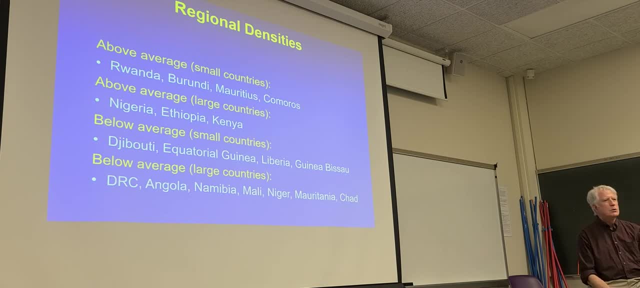 beholden to some of the ideal ideals of the past, 50 years from now, 100 years from now. i get, i get heartened by some of the progress that many of these countries have made, but i don't know it's it's still too easy to tamper. you mentioned the riches. 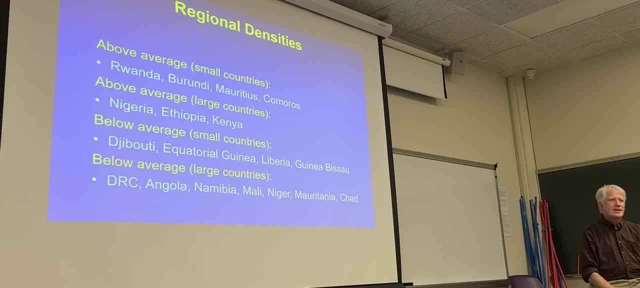 that were there. you know there's still. where are all these countries- china- i have to pick on a little bit- especially looking to find the raw materials that they need? they're looking to africa. they're looking to that africa as a bread basket, as the pantry for extraction. 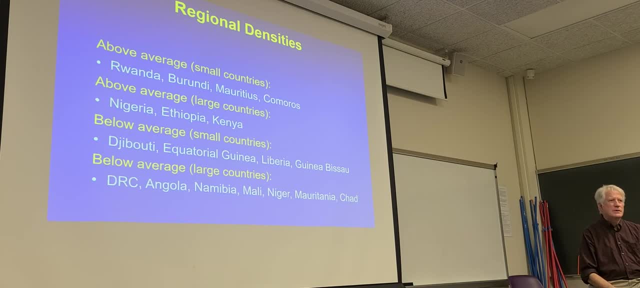 absolutely, that's something that's understood, like well understood, but also, yeah, i don't see that's where. again, i don't have a crystal ball, but i see that is where it's going to get worse. migration, the migration issue, climate refugees, migration issue- i mean it's already. i 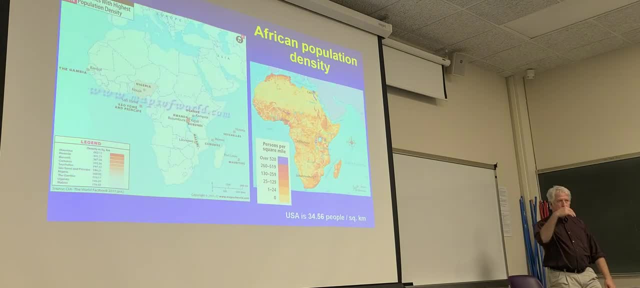 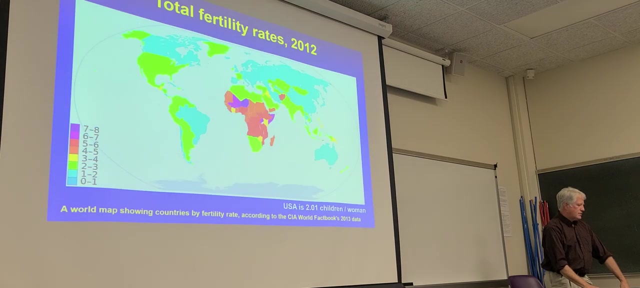 mean, if you're looking at, you know here we're giving third shots of covid vaccine now, right, boosters and many places never have been heard the first bag. so yeah, this again put density aside and start looking at some of the factors that are affecting some of this movement around. yeah, they're having high birth rates. some of the growth. 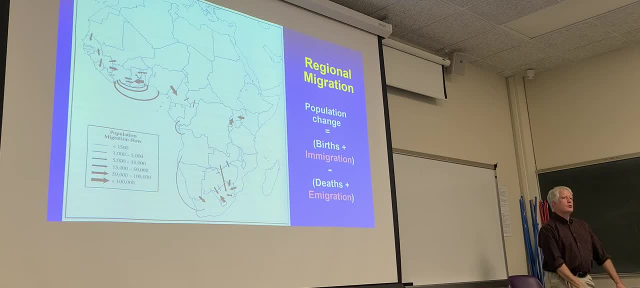 is gonna happen in africa, but it's this migration: internal, external migration. right now, i think we're seeing the effects on our southern border. you know, build the wall, make mexico pay for it? um, certainly, i think. as we've seen it, LED pays quite well, though, for instance, if you're. 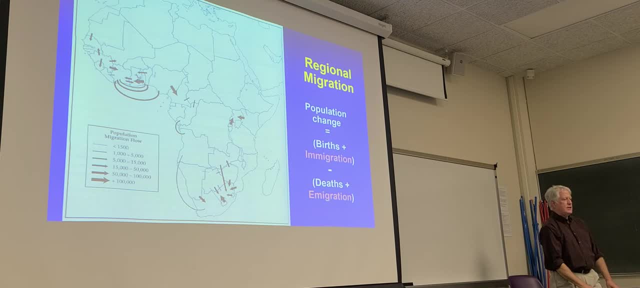 Certainly the Haitians in Texas last week, but that's just a snapshot in the news. This is gonna keep coming. And same thing with Africa towards Europe, towards the EU, Italy or wherever they happen to land. I see this is getting worse before it gets better. 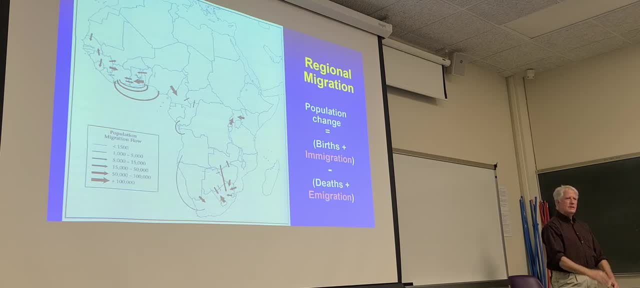 I don't know how we're gonna deal with this. Do you have any ideas? Me, Yeah. I think that in some shape or form, away within our lifetimes, within this generation's lifetimes, that there's gonna have to be something. 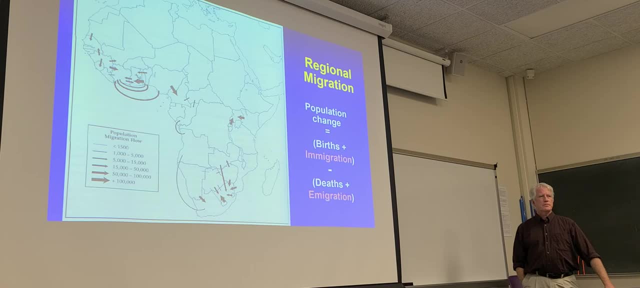 that changes drastically, Just not even from another perspective. let's just look at it from a planet perspective. We have 10 years of work left to do. Just this year, this summer, we had a hurricane come through the south and go all the way to New York. 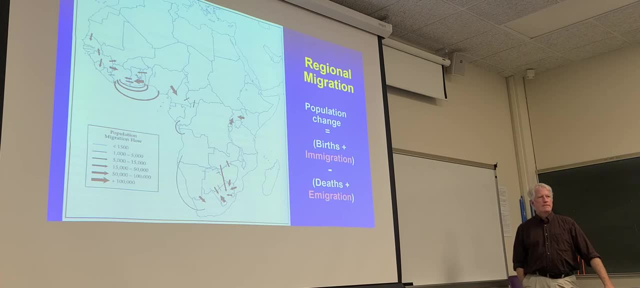 inland, and hurricanes are things that use water. they need ocean, ocean currents and whatnot, But this one was so powerful that it literally swept the whole United States. That keeps happening. Just to say, this winter we have just like last winter. we don't have that much of a winter. Winter starts in January or February, So I feel like that's really going to affect not just the United States or the Western world, but the whole world in the same way. I think you're right. 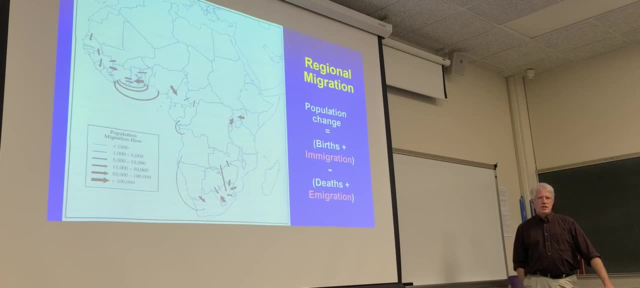 Did climate? why would somebody leave where they've grown up, where their ancestors are, where people know them? they speak their language, their culture? is there To go somewhere where they know that they're not wanted? Unless it's desperation, People don't ask those questions. 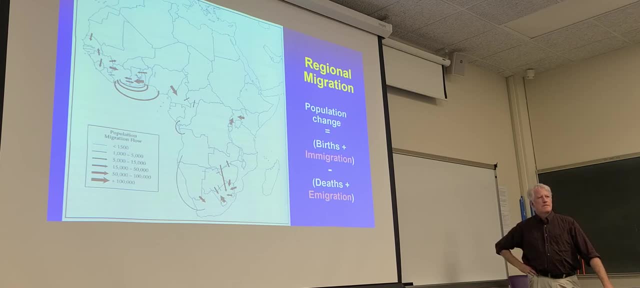 People from my perspective. I'm new to the Midwest, I've only been here three years. I go here for college, further college. I can't wait to leave. So, from my perspective, I've never experienced like a culture shock worse than this place. 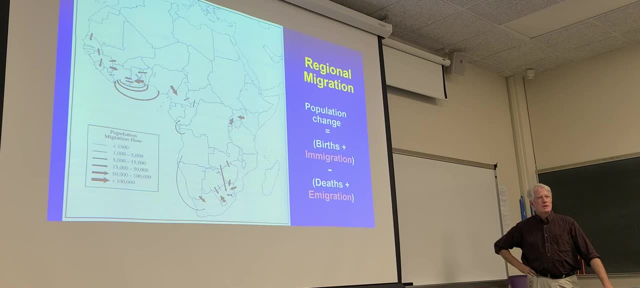 And that's because people here, for the most part they're untraveled. They don't really understand any culture besides Midwestern, I wouldn't even say American culture. They don't understand any culture. They don't understand this kind of passive aggressiveness. 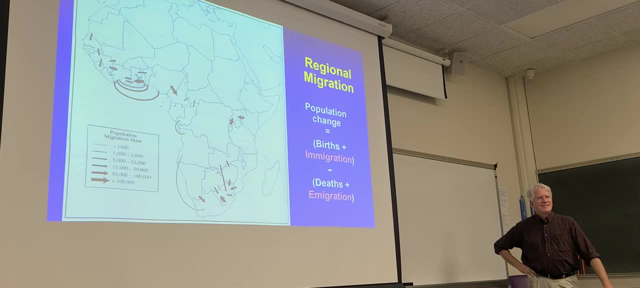 and insolvency and all this other bullshit. But just kind of going off of that, I feel like that's a question that a lot of people don't ask themselves. Why would these people leave somewhere where their fathers have been for generations, where they're from, where they speak the language? 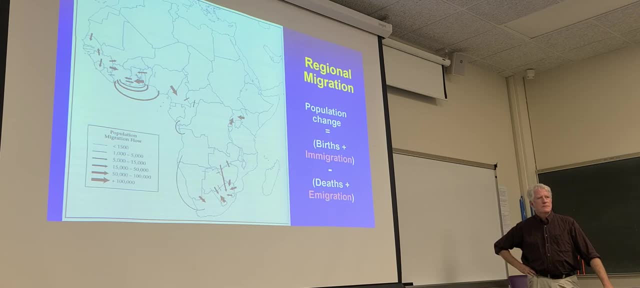 where they understand everything and come forward to seek a better life. What makes a person want to do that, What makes a person go out of his way to do that? Not just that, but what made your European ancestors- because not everyone came here on the main cloud. 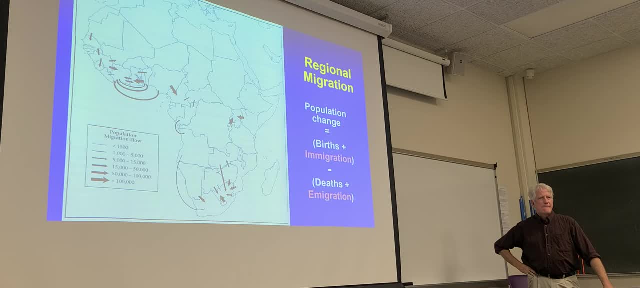 there's a lot of Scandinavians here. there's a lot of people who are from Sweden. all of that. What made your ancestors do this? I feel like people need to learn more about themselves and their history. That's true Irish. mine came here because of the potato family in Ireland. 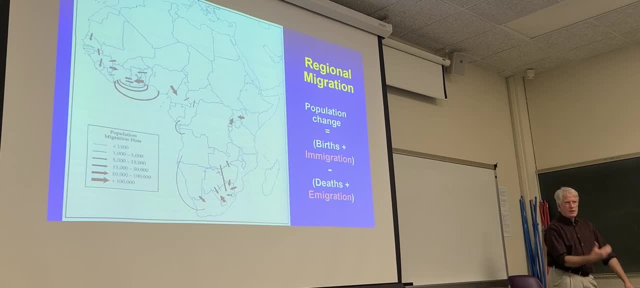 And they couldn't live there no more. They had a better life here. But when the Irish came here, it's like Irish not wanted- All right, we've got to be. And now it's blacks not wanted. Times change, Yeah, well then, Chinese or Italians or whatever. 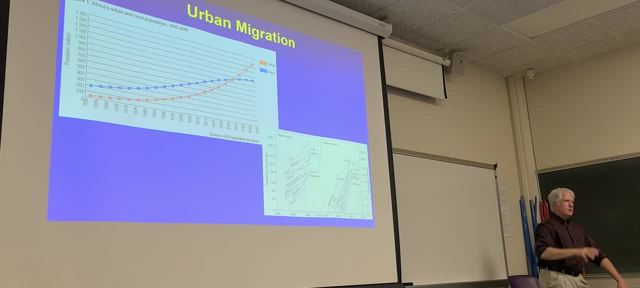 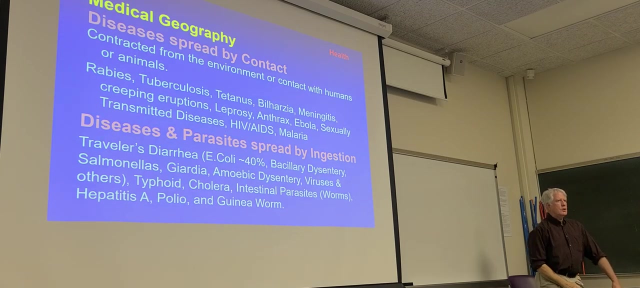 it does change. But, yeah, migration Internally, though. it seems like many people are heading for cities, just like here. right, People are heading for cities, but can cities support them? A few other. we can talk about that topic for a long time. 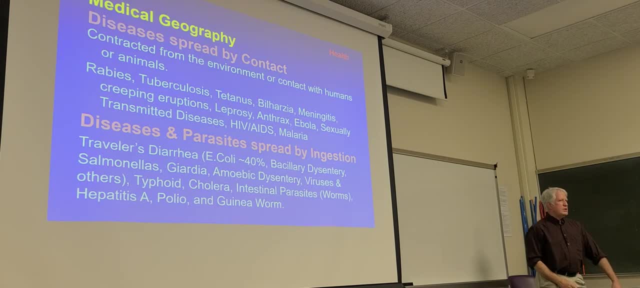 Other challenges again. it's just not a unique thing. Zika right. Zika came from the south and has its own hazards, But many diseases are identical In Africa and elsewhere. if you think about it. malaria is around the world because there's 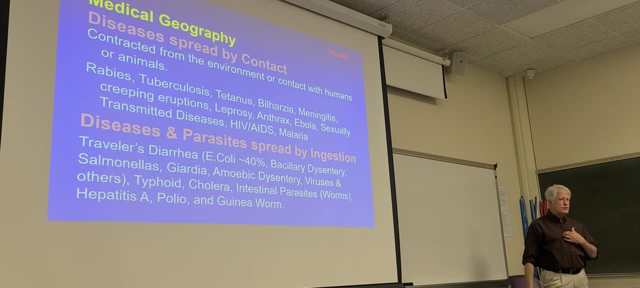 certain mosquitoes that transmit malaria. Our country doesn't have to spend money to combat malaria. We can spend money to build better hospitals or childhood vaccination programs, or roads or schools, whatever it might be. But if you have to take a certain portion of your budget, 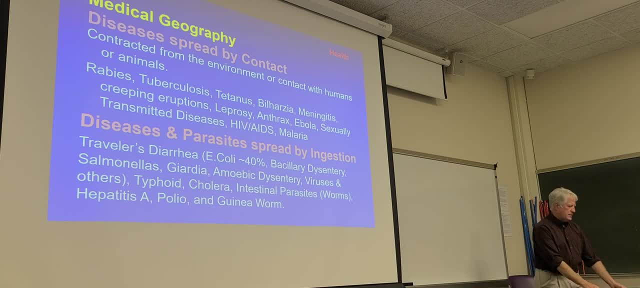 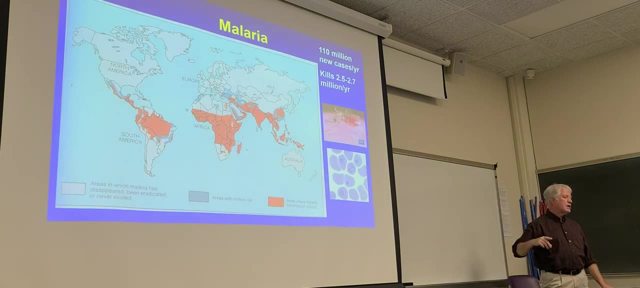 to combat these diseases, you're not getting ahead. So these are some of the diseases that are again, not just in Africa, but many places in Africa have to struggle with, And this is a big killer: It's malaria transmitted by mosquito. 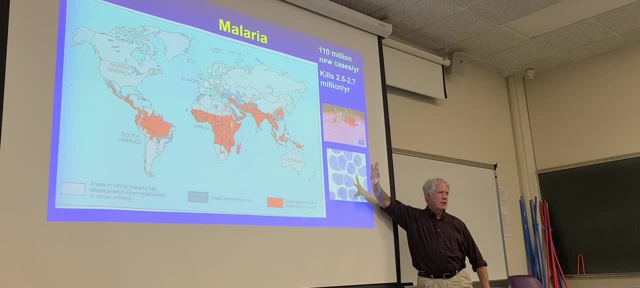 And it's a little parasite that goes in your red blood cells, which then bursts your red blood cells and you come out with fevers, chills and, in some cases, death. right. So this is where it is endemic, right. 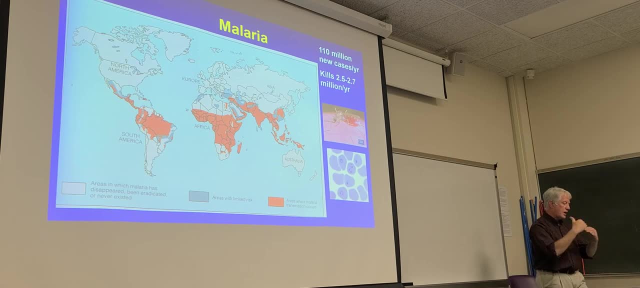 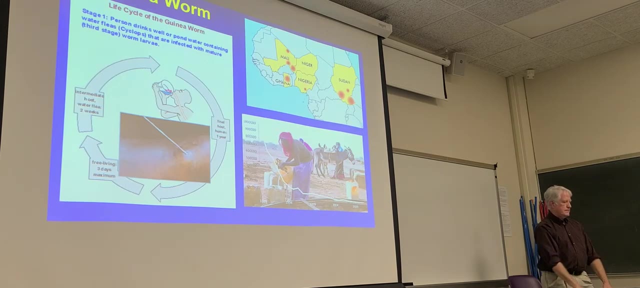 But again, this could change with climate change. Those mosquitoes could be back up in the United States, But this takes a toll on public health systems. Guinea worm: yeah, When it comes to treatment, a lot of people transmit the malaria, So a lot of people there can't you cure it in some cases. Can they get rid of it? They've been working on a vaccine for 30 years and they're still working on it. It's hard. It's not like a virus. If you're sociopathic, you get it less bad than 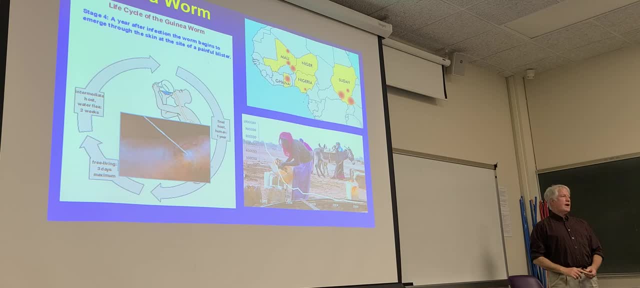 Well, the treatment for it is chloroquine phosphate. So you take 500 milligrams of chloroquine phosphate once a week. What that does: when you get bit it goes and hangs out in your liver, But when it comes out to your bloodstream, 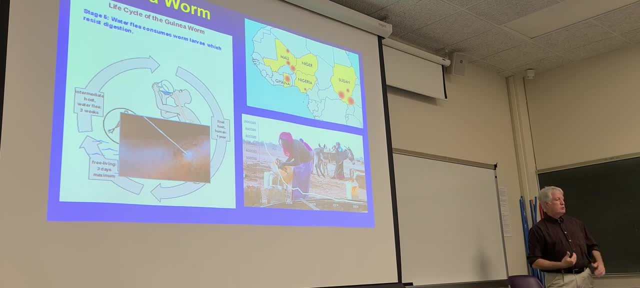 the chloroquine phosphate kills it at that stage It's still in you. When you leave a country, you can take another pill called Premiquin, which will knock it out of your liver. There's no sense in taking that in country. 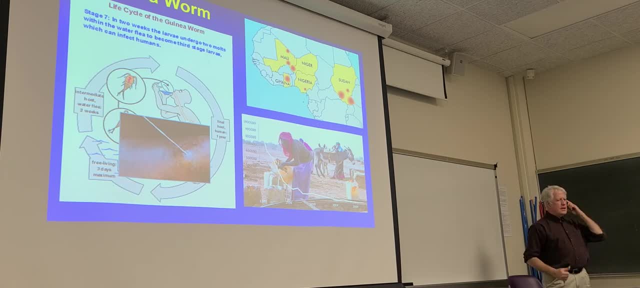 because the next occasion it'll bite you, we'll just put it back there. So it's not a treatment necessarily, but it knocks it back so you don't get the symptoms. So why, If you have access to it, Access OK. 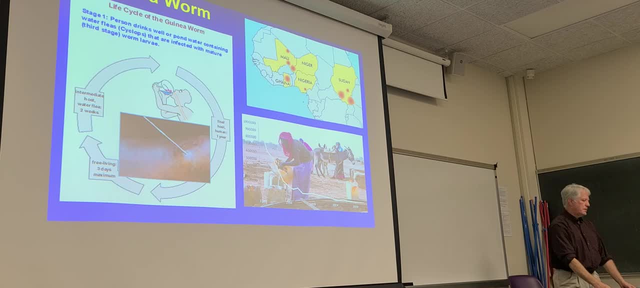 If you have access to it, And then everything costs right. And then a distribution problem: Guinea worms all swing up and bite This one is this close right, Kind of like we're this close to solving polio. We're this close to eradicating guinea worms in the population. 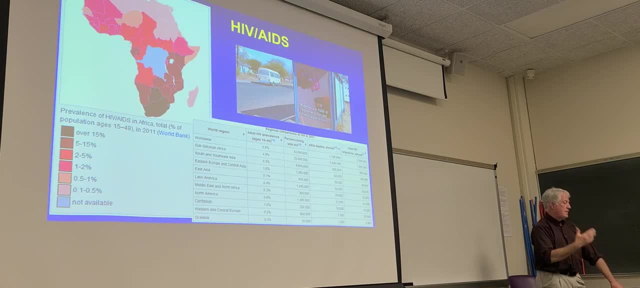 HIV-AIDS is prevalent there as it is in many countries of the world. It's thought to be a mutated green monkey virus And maybe it started there. maybe it didn't, But it's endemic in many places now. So again, 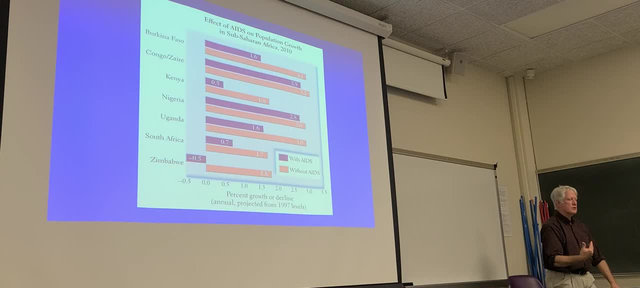 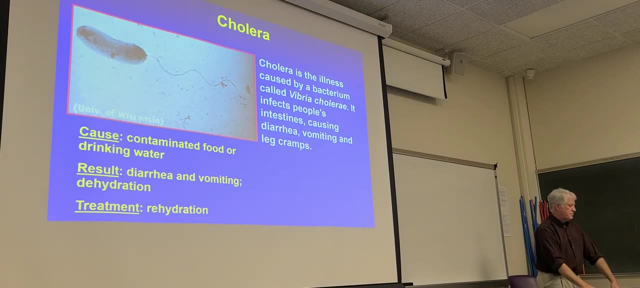 Much of this, A lot of your public health monies, are going to treating some of these things, And it could be put to better use if this wasn't on the landscape. Cholera is another thing that just kind of pops up wherever there's a container drinking water. 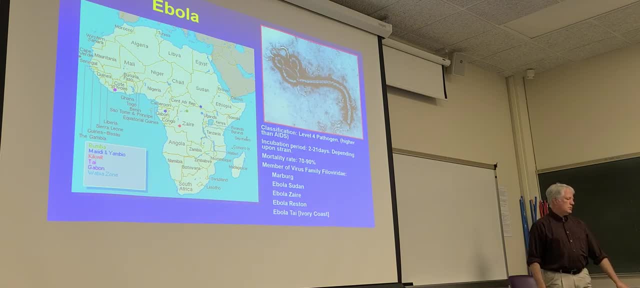 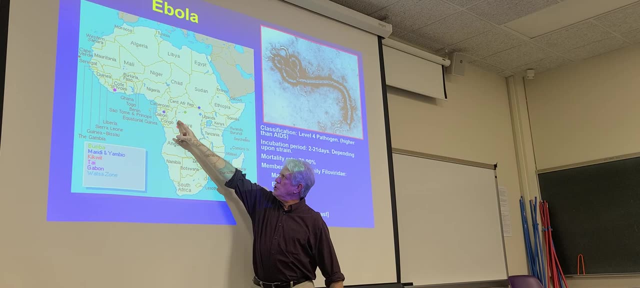 Ebola is a different thing. Ebola came from Zaire up in the Ebola region up into here. It's some of the earliest cases that it was found. It's a heinous disease. It's almost 90% fatality. It's almost 90%. 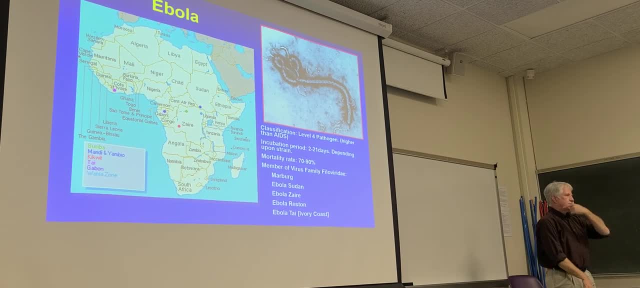 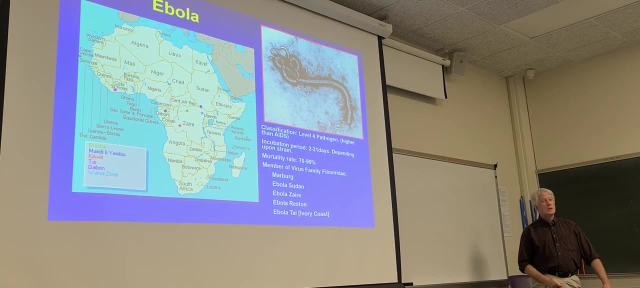 Imagine if this was COVID: it would be almost like an extinction-level event. Or if this was airborne, it would be almost an extinction-level event. It's hard to transmit, But once you get it it's hard to treat. So why didn't it spread before? 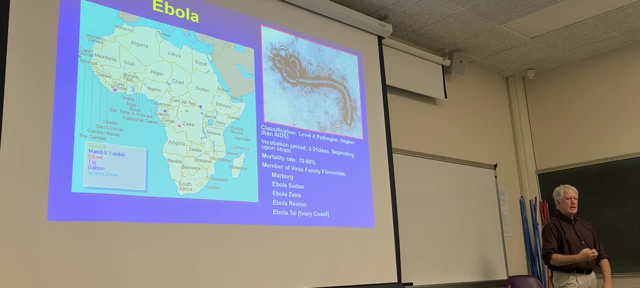 Once it flared up, it's still there. There'll be another outbreak, people, But it's not gone off the planet. It's that when you get a flare-up, nobody traveled anywhere. Everybody there that got it died and it didn't spread. 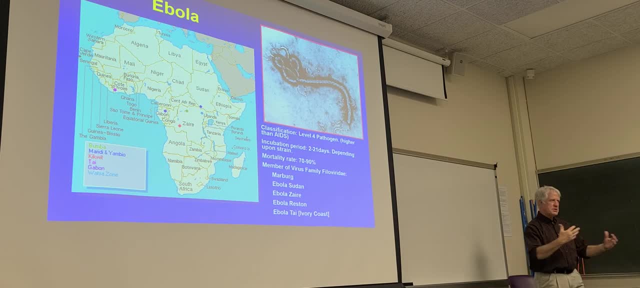 But now with international or national transportation they can get on a plane asymptomatic and spread it around. So many countries are really looking at this one as kind of the next pandemic, And if it mutates beyond this, that's much more of a concern. 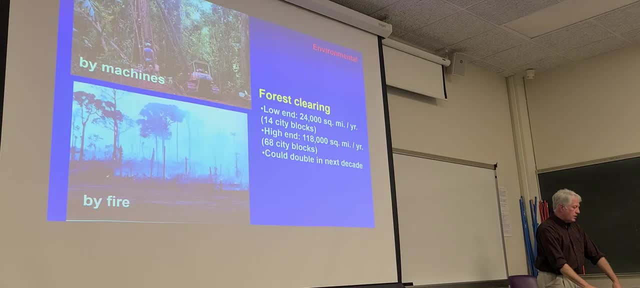 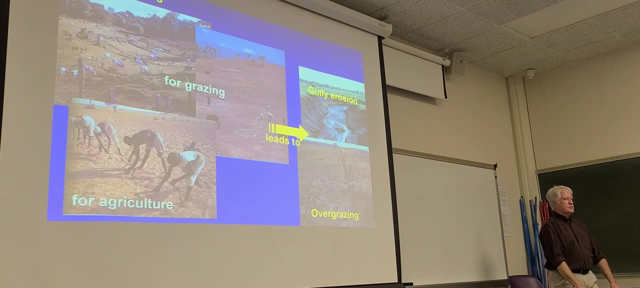 much more deadly Life expectancy is a consequence for all these things- malnutrition, environment- So we can mention environment. Forest clearing is going on Again. The Chinese are looking at this. Other countries are Certainly. many countries have for the teak, for the ebony. 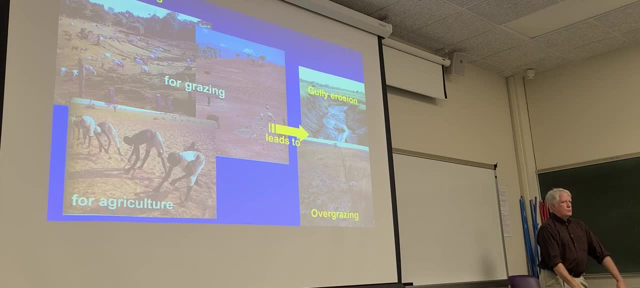 for whatever it might be. But internally, what are you going to sell on the world marketplace that the world wants? If it's something unique, you can make money. If it's not, well, every place can grow. A lot of places can grow corn. So that's not that unique. Some of these countries, especially in the landlocked, need money. One of the ways to get money is through tourism, ecotourism. Back in the day it was like elephant hunting. Go shoot an elephant or a lion hanging on your wall. 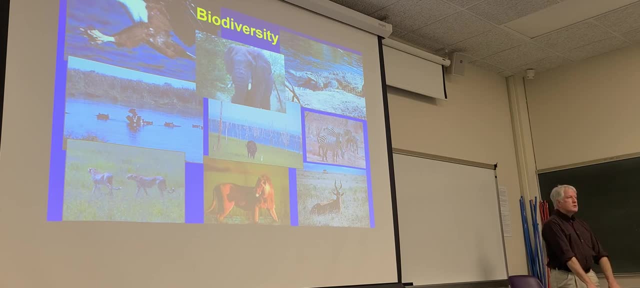 Now it's more. take pictures. So people know this And ecotourism is a big business. You can go there and everybody in the local community profits from people. You can go to Australia. That's a long ways to go. 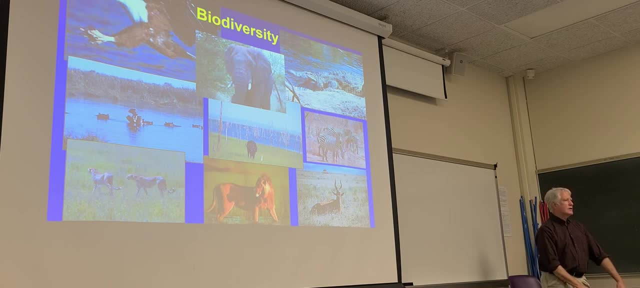 What are you going to see? You're going to see- good luck trying to see a platypus Or a guava- right. You go to Africa. you can see all these big things, right. There's nothing unique about North America. 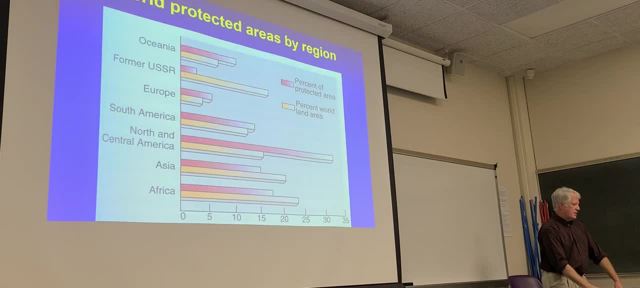 that people are going to come here to see. But Africa, yeah, they get some money in there for hard currency, So they're very well protected. Some of the biggest and earliest world preserves on the planet were in Africa. There were some very well-established national. 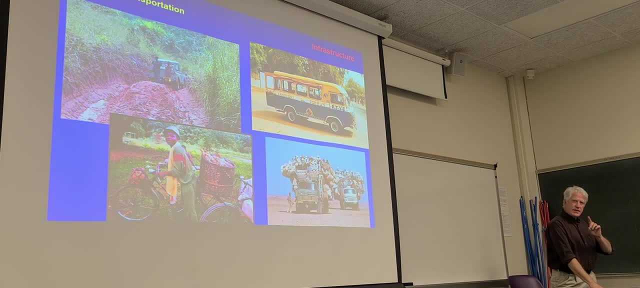 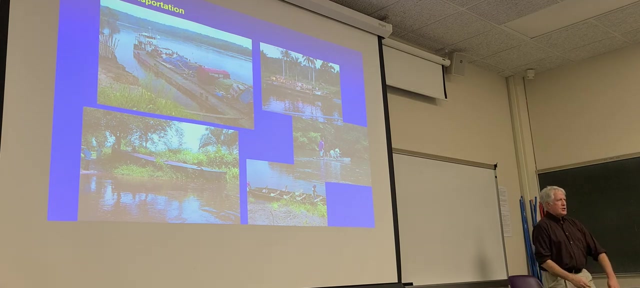 harps here. This class ends at 40 after. OK, a little bit more Transportation. It's not a challenge anywhere, even here in Minnesota. Getting things around roads are great, But harsh rainy season conditions can turn them into peanut butter, like the one on the top left. It's hard to get around. Public transportation is good in the large cities. River systems- either small canoes or barges- are perfect because you don't have to maintain that There's no money that has to be spent. And we'll get to this last one. 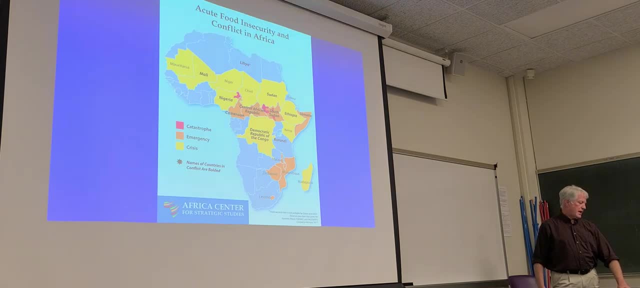 And unfortunately, we end this with. what do you call this conflict? Some of this conflict are legacies from colonial times. Some of those are external. Some of them are internal- old grudges, things like this- But there's still some food insecurity here. 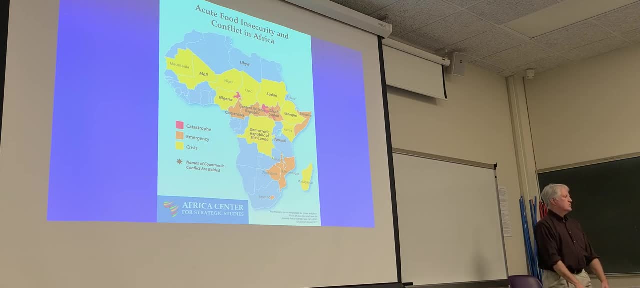 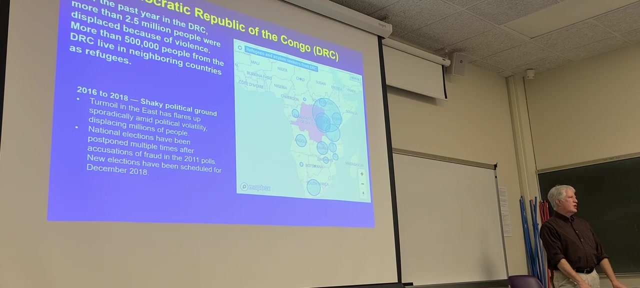 And you're going to fight over natural resources or water-loving food. I would have to say that much of the world is much safer than it has been. There aren't any world wars right now, but there are still some internal conflicts. This is one that's in DRC- Democratic Republic of the Congo. 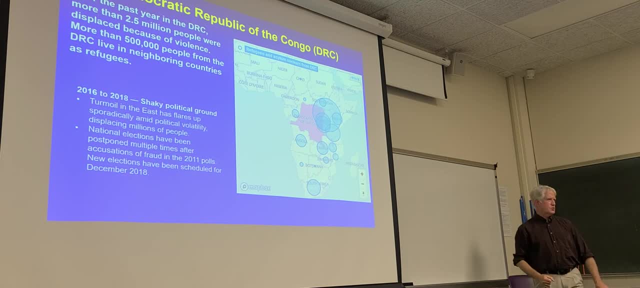 It's a huge nation, spancy, equator. It has just about everything that you would want. It's got unique things like Bonomo chips, okapis, mountain gorillas. It's got gold. It's got timber resources. It's got great agricultural potential. 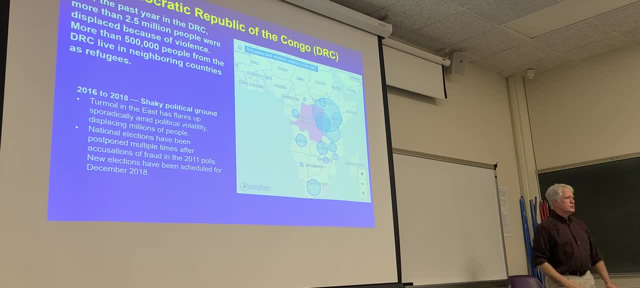 Wonderful culture. If you go to any museum, they're just going to have representations from music, culture, painting, carvings, et cetera. dance from the Congo. But Eastern Congo is almost. it's a very troublesome place right now with a lot of rebels around that particular region. 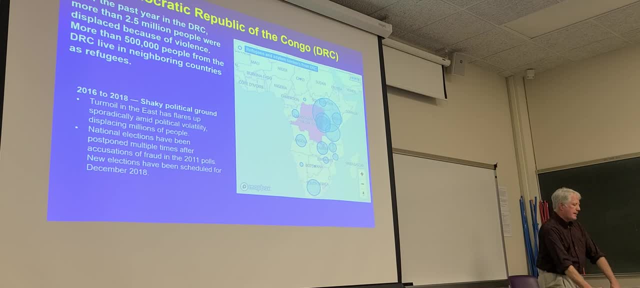 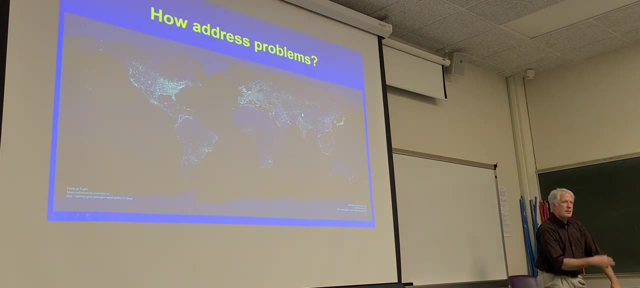 kind of hanging out and causing shaky political instability. The capital is Kinshasa, over in the west, and it's very hard for them to control everything in the east. How do you address these problems? This is a shot from space. We look at this and say this is where people live. 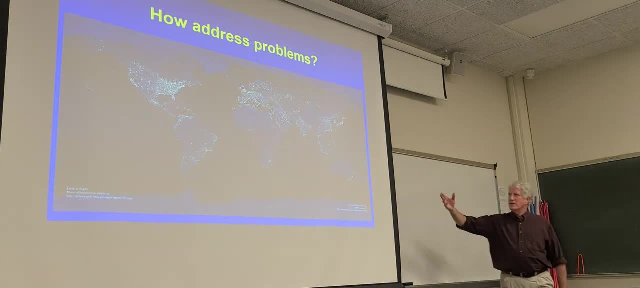 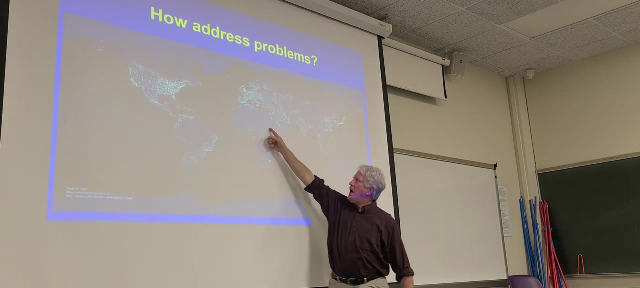 That's what I would say. This is where people live, But we know that there is, I mean, not a lot of people in the outback of Australia or in the rainforest, but we know there's people in Africa, It's just that they are not on the electrical grid. 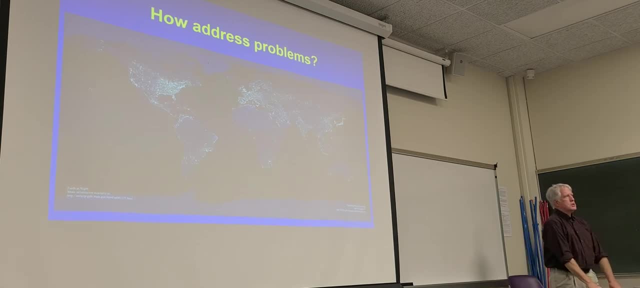 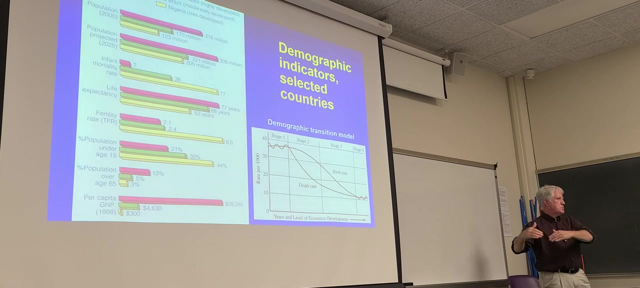 Not very well anyway, so they're not well represented. How can you economies go forward if you don't even have an electrical grid, which means no lights at night, no electrification, no factories? So some of the demographic transitions if you can pulse through as fast as you can. 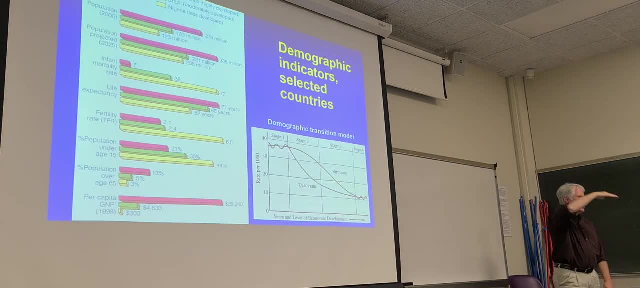 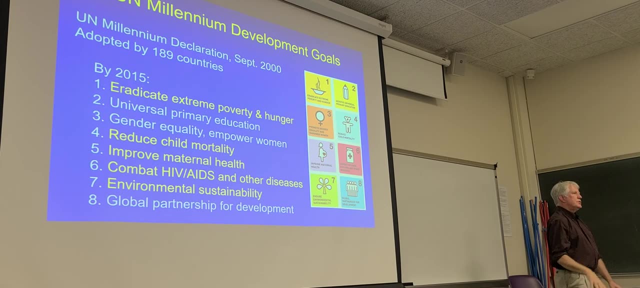 most countries are up in stage three. So Birth rates are coming down, Death rates are coming down. They're getting a little bit richer, a little bit better. The UN came out with Millennium Development Goals in 2000,, a 15-year plan to get less economically developed. 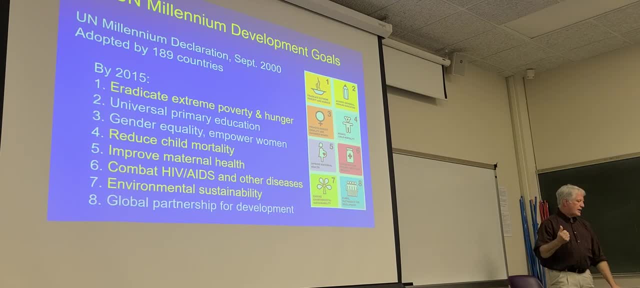 countries basic needs met. One: eradicate extreme poverty and hunger. Four, five and six: child mortality. improve health, HIV, AIDS and environmental stability. You can imagine this is across the board, across many different nations. Right, It's 15 years. 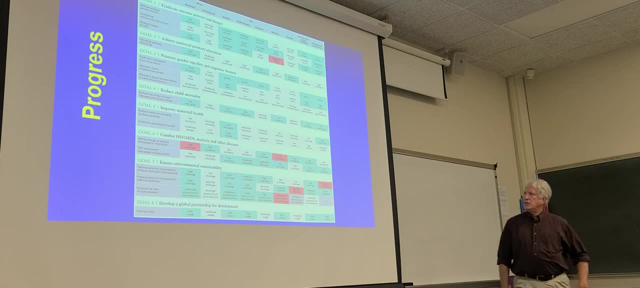 They reassessed how we're doing And unfortunately the red very low, moderate low incidence et cetera. here Asia the gate, Africa, sub-Saharan one, Very high poverty, very large deficit, high hunger. 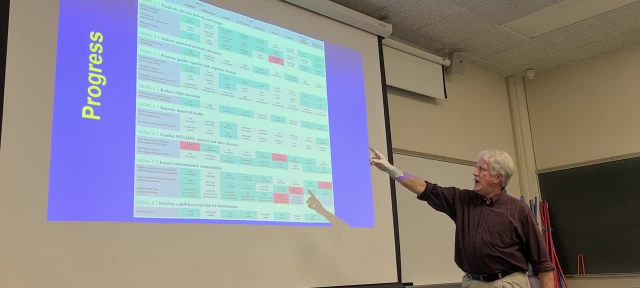 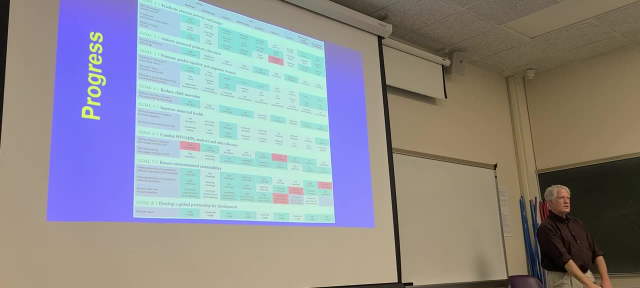 down to four and five: High infant mortality, high mortality, low access to reproductive health. They could do better. They came back in 15, reassessed The next plan that we're in right now. they, of course, increased the number. 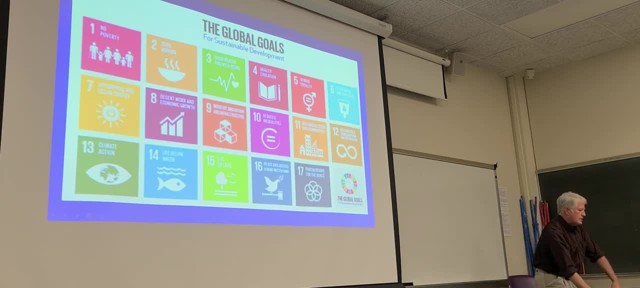 And, I think, a little bit aspirational. here is no poverty, zero hunger. That's a big ask. right, That's a big ask, But this is aspirational, perhaps. So this was 2015.. We're now in 2021.. 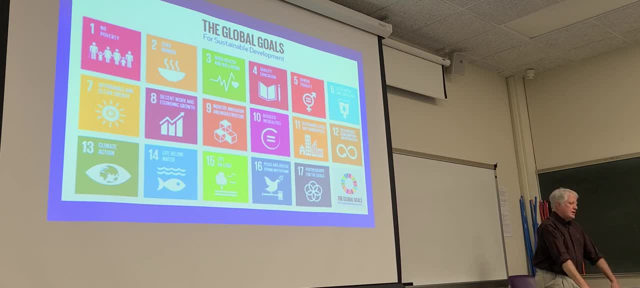 So we're quite halfway through, But I would hate for us to get to the end of this and have to do another 15 of the same ones again. There's no progress that's been made, But again in 15 or 20 years it's. 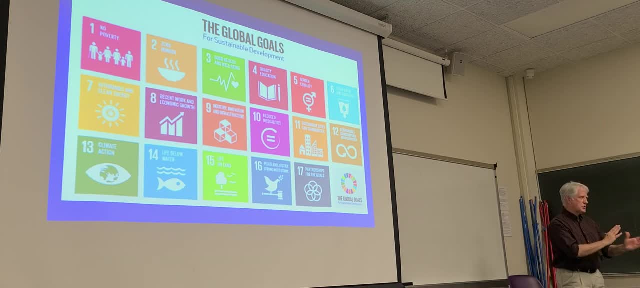 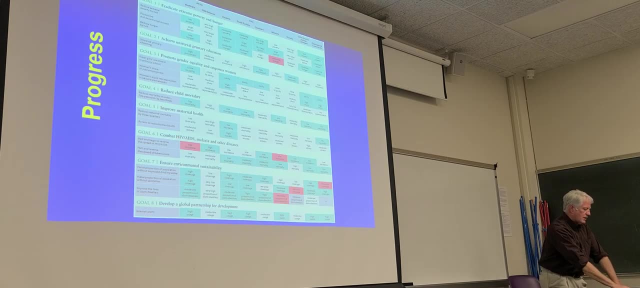 hard to turn back or hard to change some of these. You don't turn a battleship on a dime, So it's hard to change some of these, But at least it's aspirational. So the UN is very cognizant, I think. 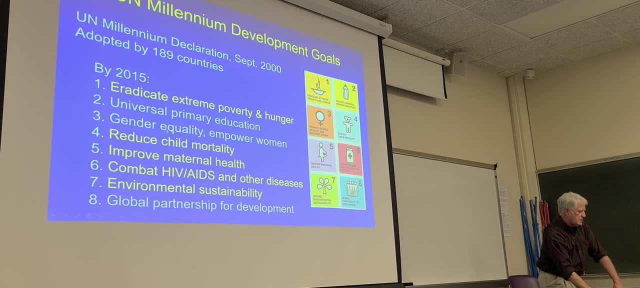 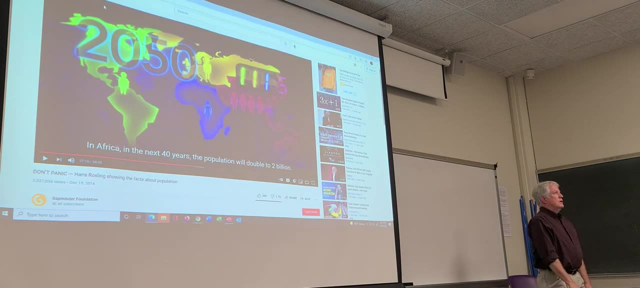 of trying to meet some of these goals, especially these for child mortality and infant health. So that's my perspective. Africa in a nutshell, Africa in an hour. All right, You're going to go into this in more detail this semester. So, yeah, thank you for all your comments and catch you next time. 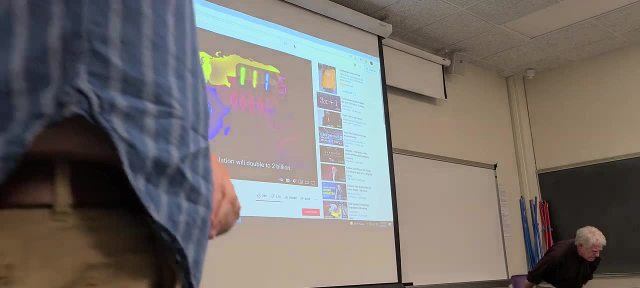 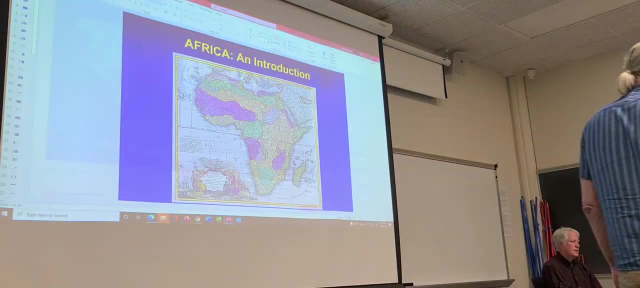 All right, thank you, Say. if anyone did not sign in, you know your 10 points. you do every day. I'm just saying you sign your name. So today, sign your name, You'll get your 10 points. I wanted to be able to get a few questions for everything. 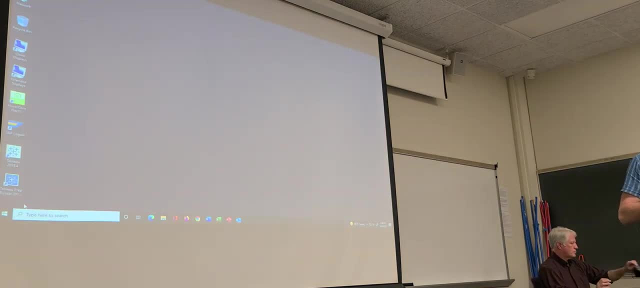 I'll just leave this here. I think a couple of people came a little late. I'm going to let them head back. I'll just let them get to this one later, All right? OK, All right, Thank you. Thanks, folks. 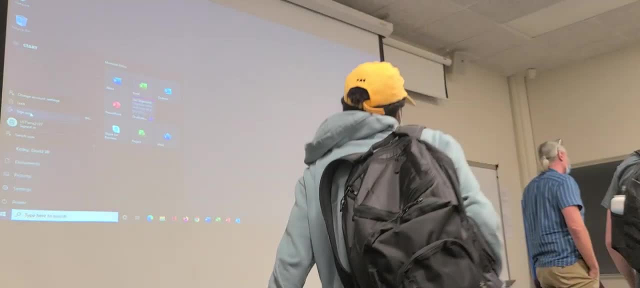 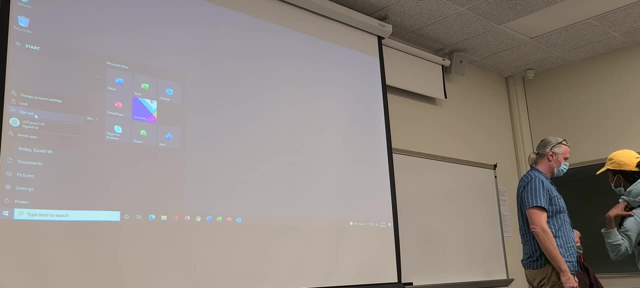 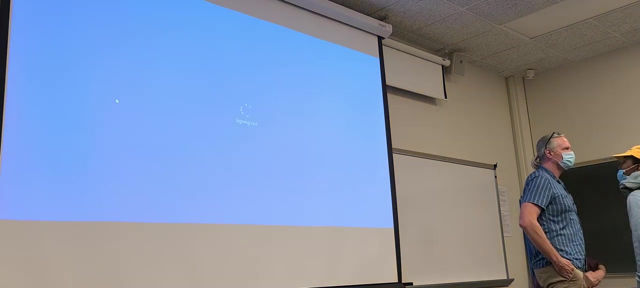 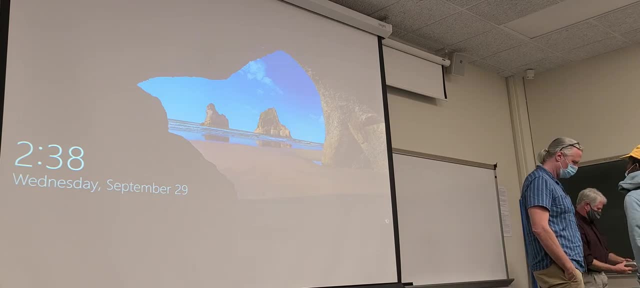 All right, See ya. Yeah, but you're being all nice because it caused a lot of problems. It's just that it's happening. There's still like around the day. Yeah, It's like the Even like the Germans like, and people still. 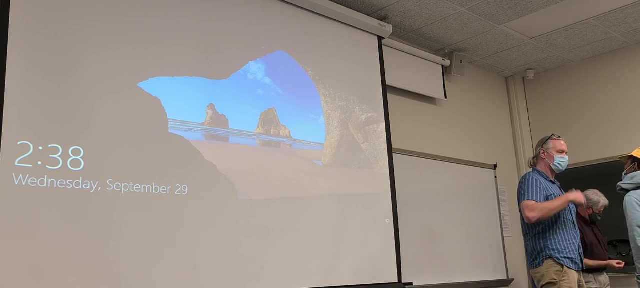 Oh yeah, you can just do this stuff. You know the questions we do. You can just do it in the center to me. so Can you tell me what dates you didn't come and I will look up what we did.